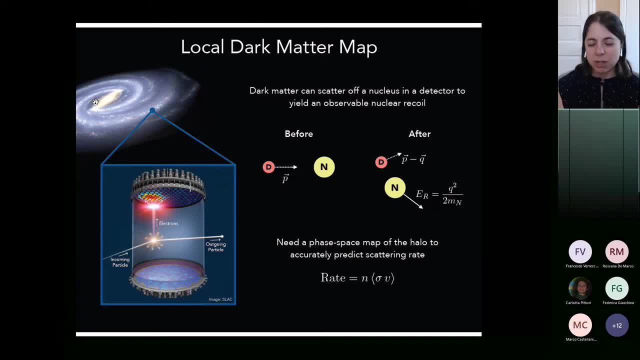 under a mountain And the dark matter particle you would never directly see, but you could potentially see its recoil effect on a nucleus or an electron that it collides with inside the detector. So these kinds of experiments are ultra sensitive and looking for these sort of small 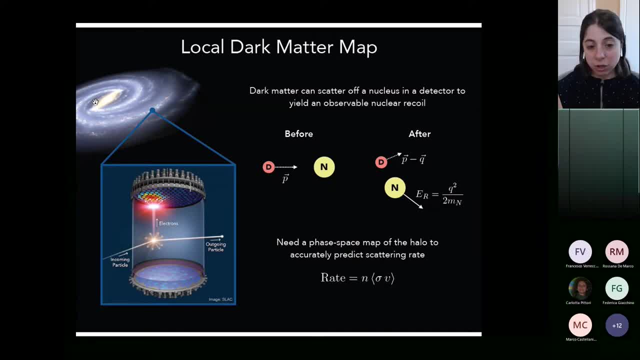 jiggles that you might see in the dark matter, And so I'm going to be focusing on that. So I'm going to be focusing on the target material that come from a collision with the dark matter particle, And in interpreting the results from these kinds of experiments, you need to have a 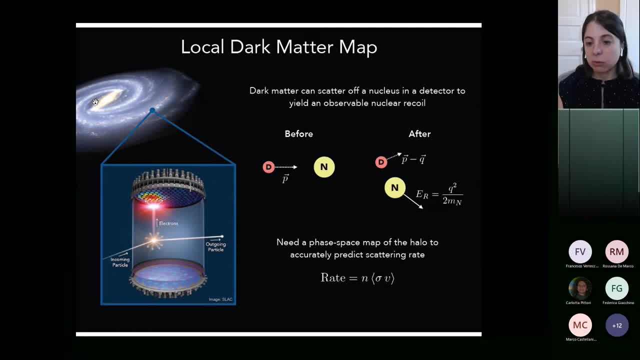 face-based map of the dark matter halo in order to predict what the scattering rate should be in the experiment. So this means that you need to know both the local number density of the dark matter- so that would obviously be related to its local density- but also its velocity distribution. 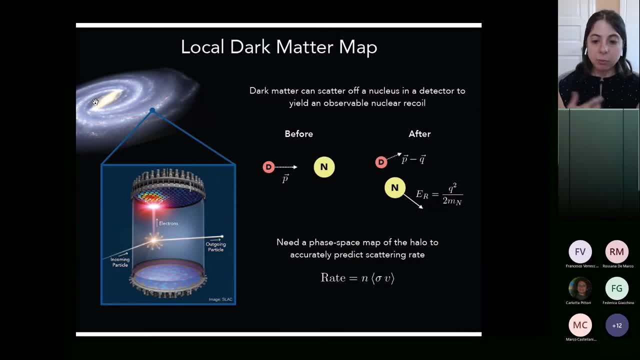 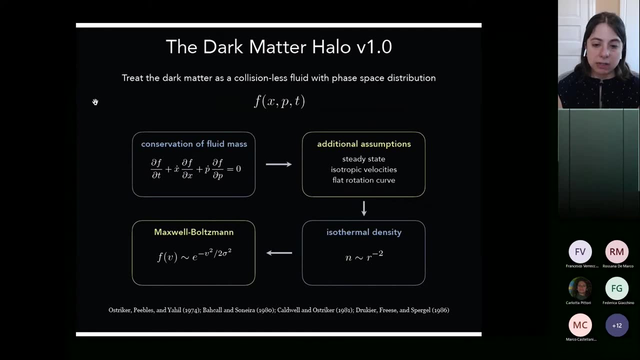 near the sun, And both of these points have been appreciated really since the very first proposals for these kinds of terrestrial direct detection experiments were put forward in the 1980s Next slide. So one of the first papers on this by Ducreier, Fries and Spergel recognized the fact. 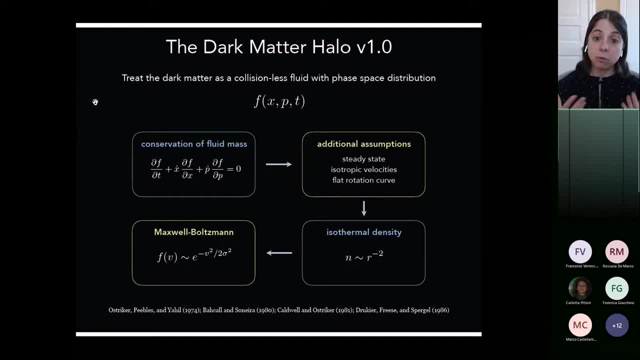 that interpreting the results from these kinds of experiments would rely on knowing information about the dark matter halo, And so they had to posit a model that could be used for interpreting the results by experimentalists in interpreting their results, And the model that was posited at that time is sort of very simple and it's outlined on this slide. It treats the 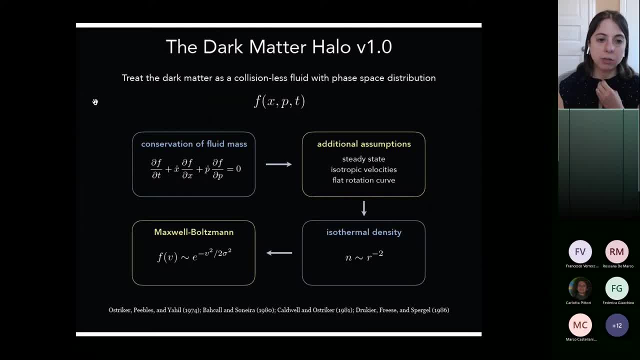 dark matter as a collisionless fluid and you assume that the fluid mass is conserved. You also assume that the dark matter is in steady state, that its velocities are isotropic and that you end up getting a flat rotation curve. So that would essentially be making sure that the dark matter is 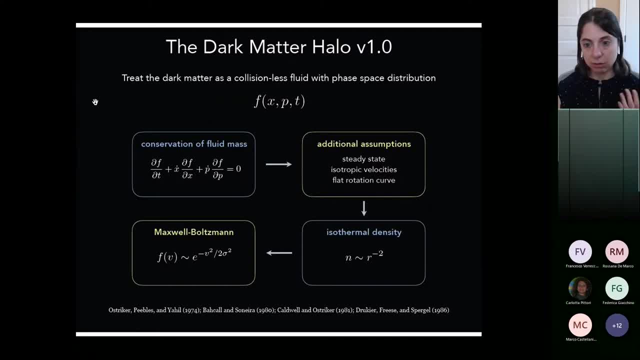 consistent with the observations, the flat rotation curve, And when you combine these sets of assumptions, it's actually quite simple to end up getting a prediction that the dark matter density locally should follow an isothermal profile. so going as one over r squared. 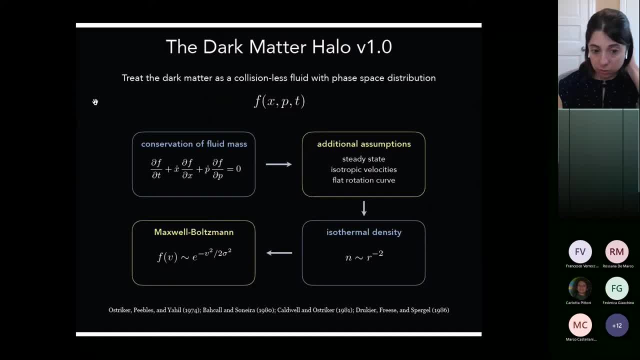 and that its velocity distribution should be a Maxwell-Boltzmann distribution. And these are essentially the assumptions that are used in all analyses of the sort of standard assumptions that are used in the analyses of direct detection experiments. So if you ever end up seeing a limit plot from one of these experiments, 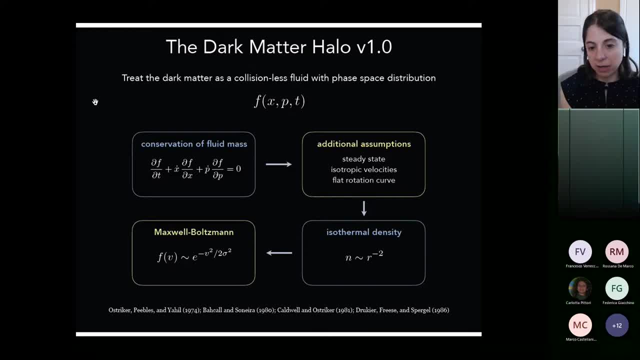 boiled into that limit line is essentially this model of the local dark matter And because it's become sort of the paradigm for what everybody uses for interpretations, it's referred to as the standard halo model. Next slide: We have an opportunity now to revisit this. 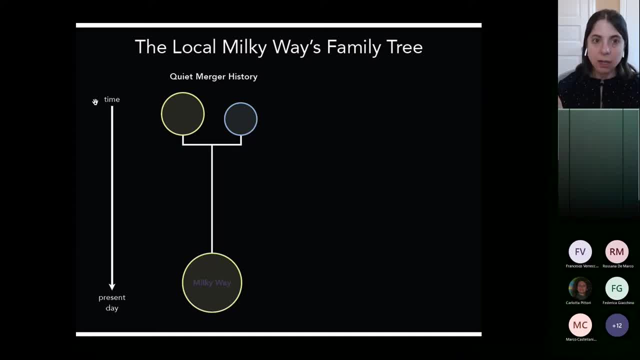 model and ask: how accurate is it? Is it consistent with the actual data? And so we can revisit specific assumptions that go into that model. So, for example, the fact you know the assumption that the local dark matter is in steady state. 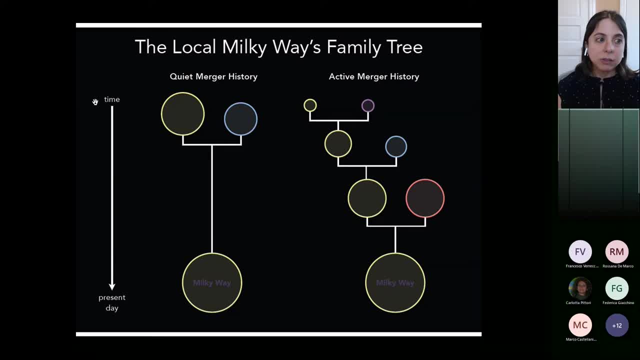 What does that actually mean in practice? That's actually a statement on the historical evolution of the Milky Way galaxy itself. So let's think about how the milk, the dark matter near the sun, actually got here. It got here through a process in which our galaxy 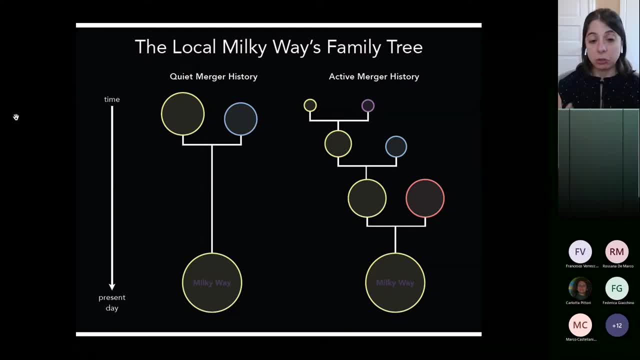 grew by accreting other smaller galaxies. So this happens over the process of many giga years And there's a variety of possibilities for how this can happen. So, for example, on the left, here is a scenario where the history of how the Milky Way evolved would be. 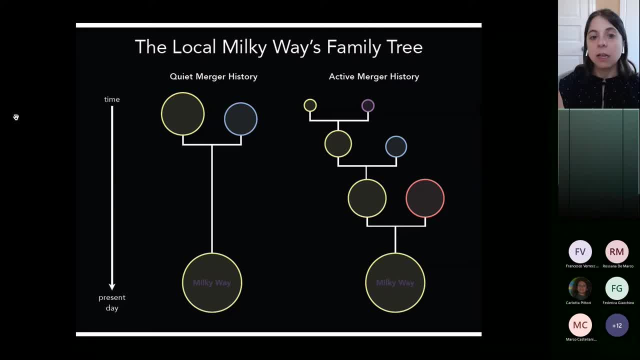 pretty quiet. So early on you might have two smaller galaxies that merge together and then just kind of sat there in isolation for a long time until you get, you know, the galaxy our Milky Way today, And you can contrast that with a much more active history where you have a bunch. 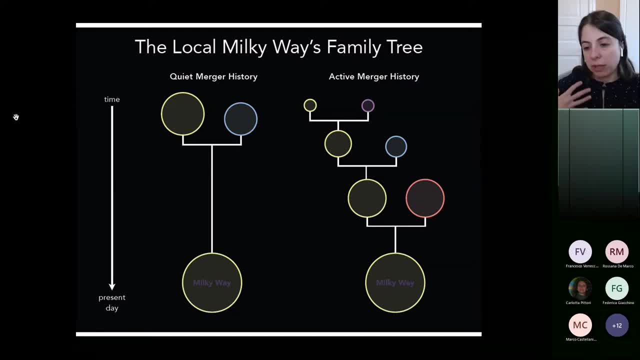 of small galaxies constantly merging with our, with our own, up until the point of the present day. And so when, when we, When we make it that stop at, and I could wings. the 16th and 19th quarter 10th. 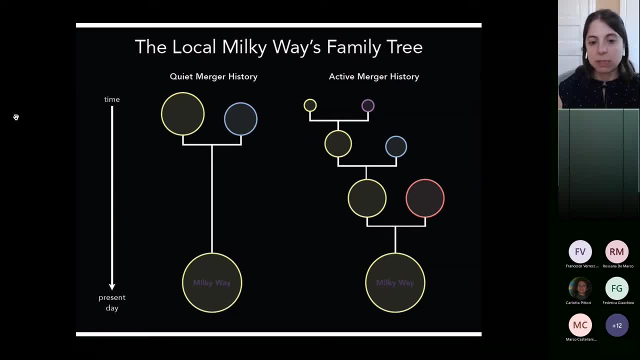 the assumption that the local dark matter is in equilibrium, that it's in a steady state. we're really saying that the merger history of the Milky Way is the scenario on the left, That's, one where the system has had enough time to come into equilibrium after the initial merger. 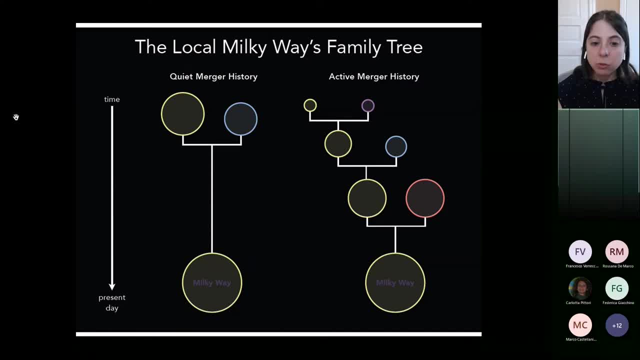 happened many, many years ago, And so we have an opportunity now to essentially test this hypothesis, because data from the Gaia satellite and, in upcoming years, from Roman and DES are all shedding light on the merger history of the Milky Way, And so they're giving us an actual picture of 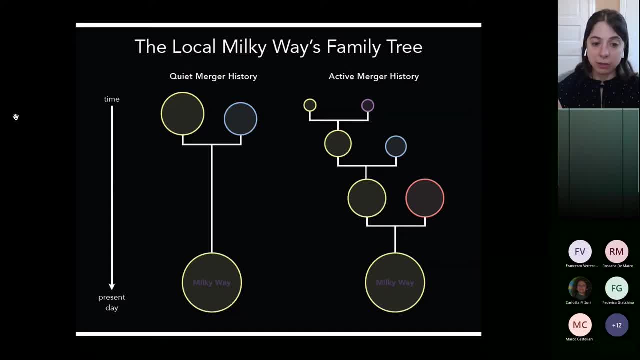 what this family tree should look like, And we can use that, therefore, to sort of understand how the dark matter near the sun is actually behaving and whether or not we get something that's that's an actual Boltzmann distribution, or whether or not it's different. 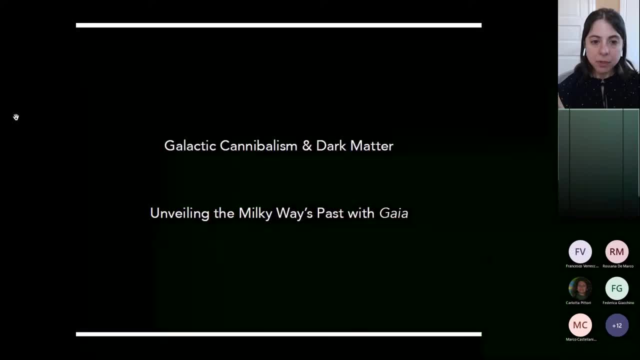 Next slide. So over the course of the talk, I'm going to start in the first half just kind of walking through this process in a bit more detail, sort of what happens when one of these smaller satellite galaxies merges with the Milky Way, gets disrupted, gets ultimately eaten up by our galaxy. 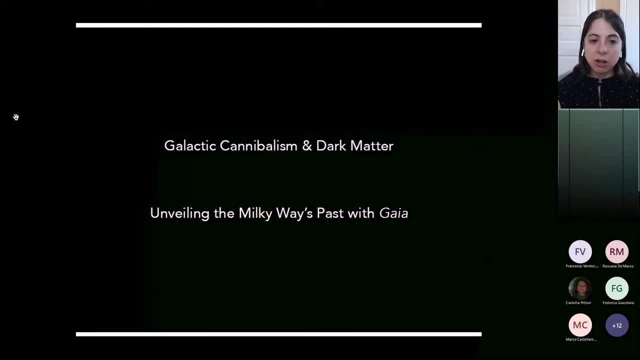 So that's why it's referred to as cannibalism, And I want to talk in that about what's happening to the dark matter. So I'm going to start with the first part of the talk, which is the data that we're going to be taking from the Gaia satellite, And then I'm going to talk about 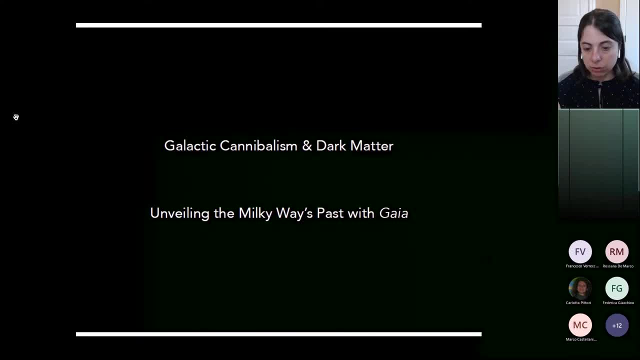 the data that we're going to be taking from the Milky Way, And then I'm going to talk about the data that we're going to be taking from the Gaia satellite. So the first part of the talk will rely heavily on results from simulation. Then in the second part, I'll talk about recent results. 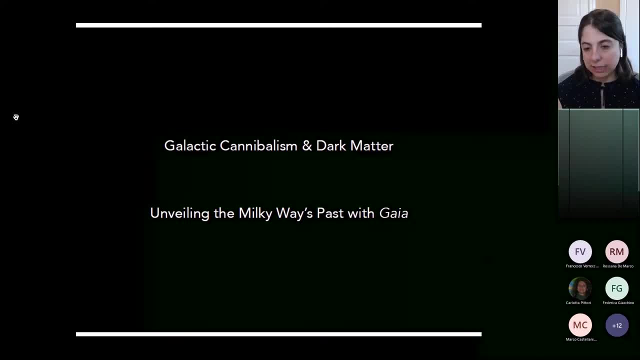 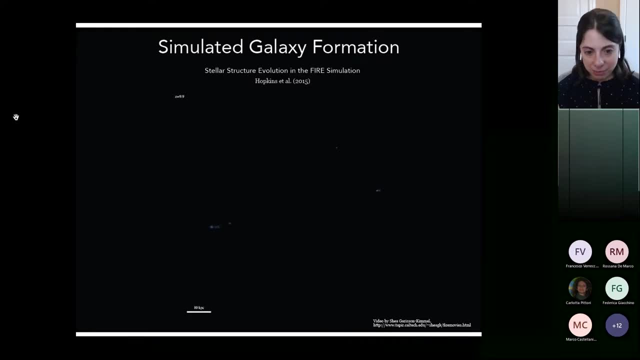 with data from the Gaia satellite, what we've actually been learning directly from the data about what's going on in this merger history and how we can tie that in with our understanding of the dark matter distribution Next slide. So I'll tell you what this was supposed to show. This was a movie of a galaxy from 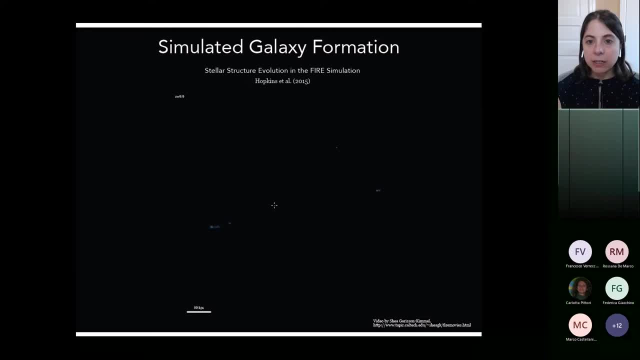 the fire simulation from a fire simulation. So fire is a hydrodynamic cosmological simulation. It's a fire stands for feedback in realistic environments, And this particular movie I was going to show focuses on a galaxy that's similar to the Milky Way. It starts at a very early redshift, so redshifts of 10.. And you can see how the Milky 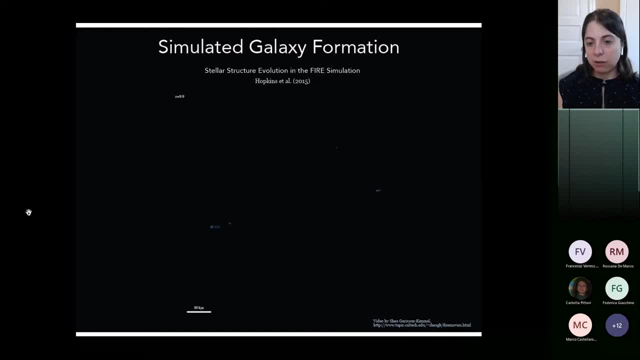 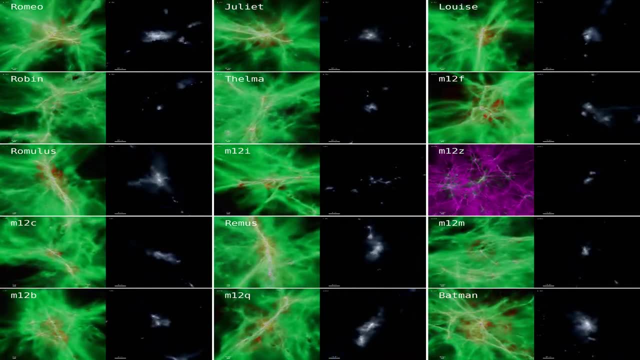 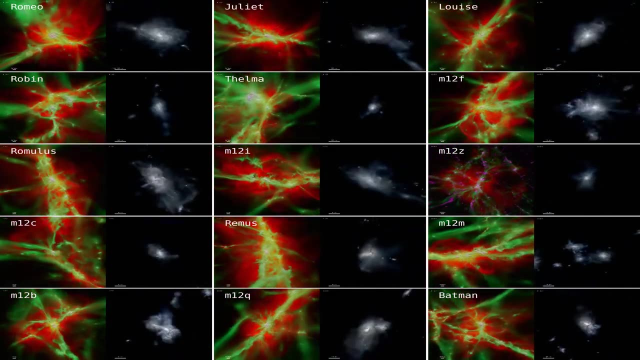 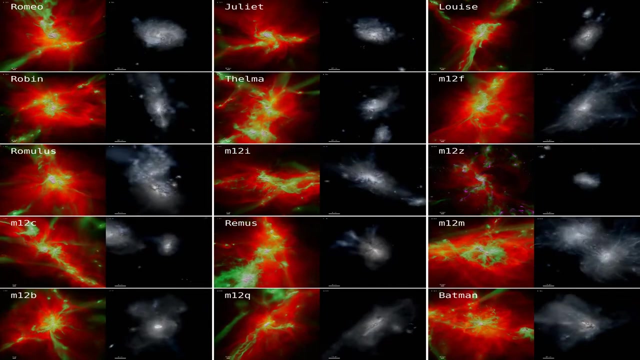 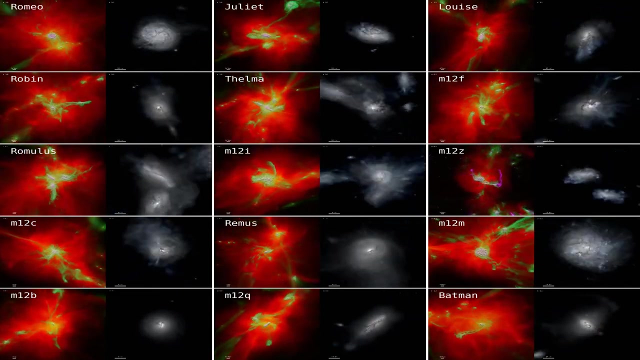 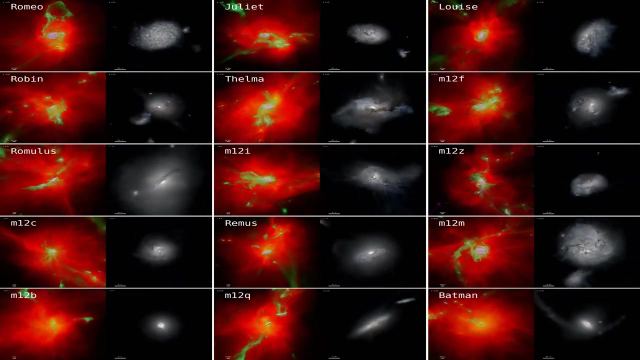 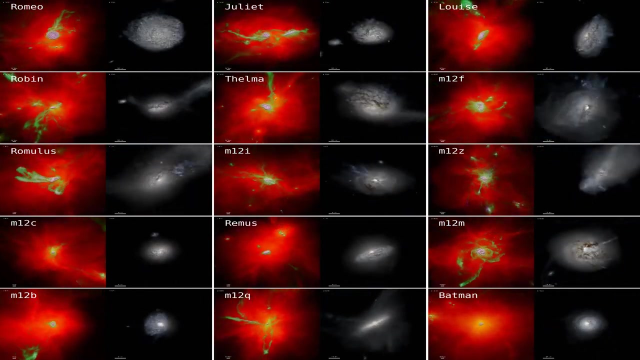 Way grows by the merger of all of these smaller satellite galaxies. So we're going to call it the Milky Way, right. So we're going to call it the Milky Way, right. So now you can look at it this way: If I look at this video from the pre-data point and if I go back to the beginning, 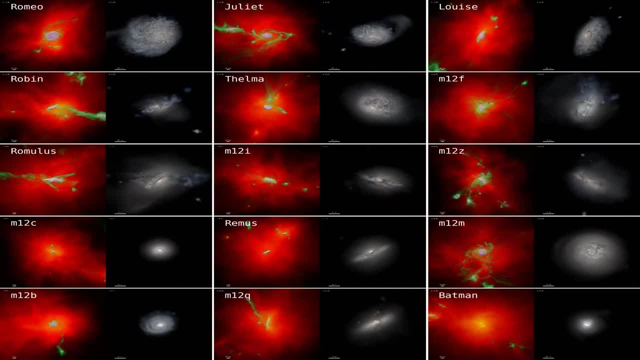 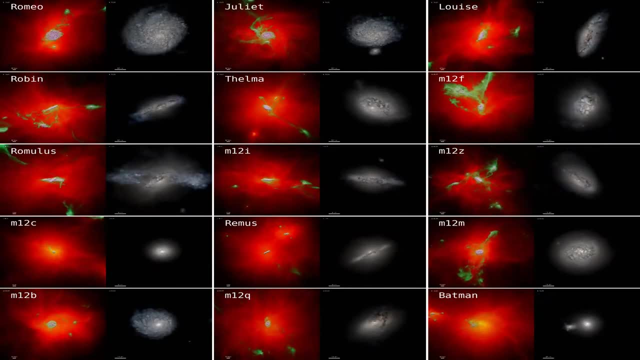 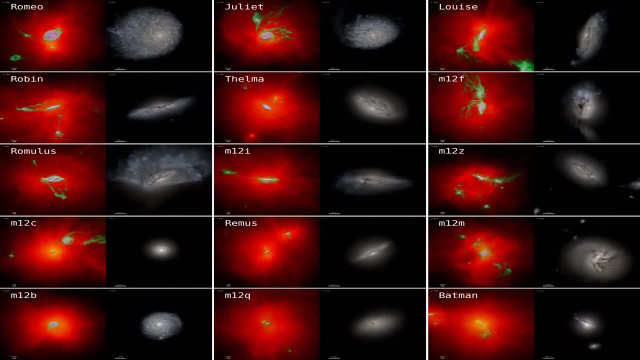 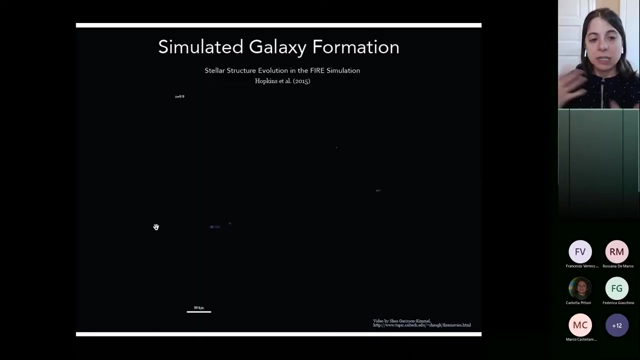 I can see the same thing, The galaxy that we saw from the Milky Way, and in the initial phase things are sort of very uh, chaotic. the collisions are very violent, but as time proceeds, um, you end up seeing that, uh, the collisions, the sort of galaxies that are. 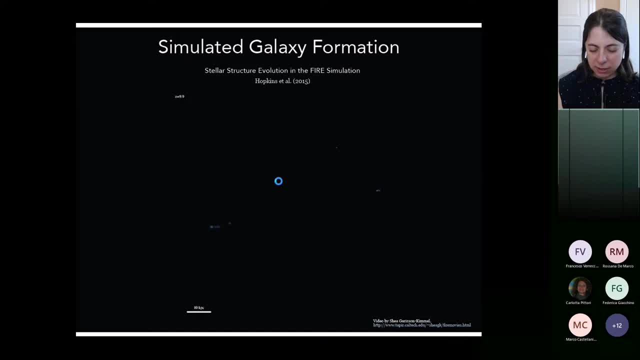 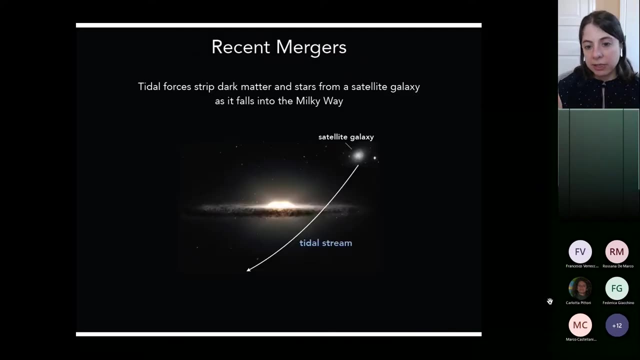 merging become smaller. um that allows for a stable stellar disk to form in the center part of the milky way, and you ultimately end up getting something that looks like the galaxy that that we see today. um next slide, uh. so let's kind of walk through this step by step. so, starting from, 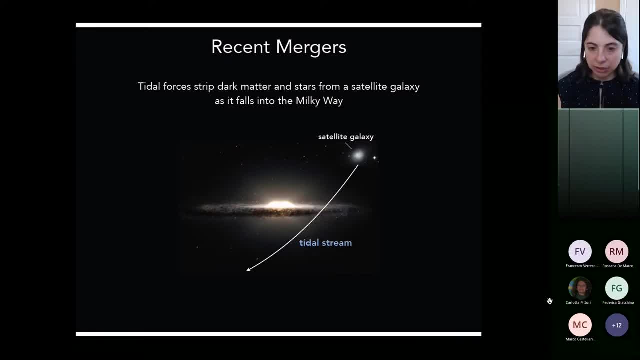 a host galaxy which we'll assume is sort of roughly the size of the milky way, and that's uh illustrated here by that, that primary stellar disk in the in the center, and we'll imagine that there's some smaller satellite galaxy that's falling in um as that smaller satellite galaxy. 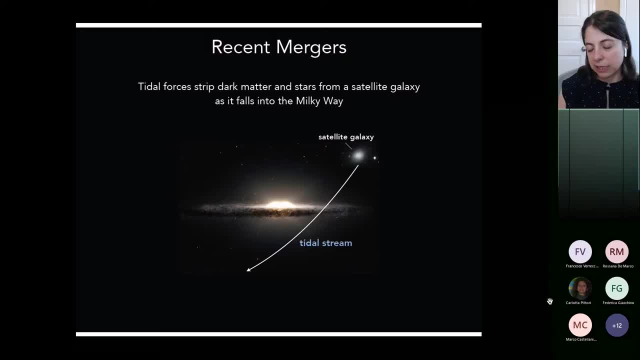 falls in, there's a variety of stages through which it's going to get disrupted. so in the initial stages, um, tidal forces start stripping dark matter and stars from the satellite galaxy and that dark matter and stars essentially end up getting left behind along roughly along the orbital path of the galaxy um. so the, in this stage, the material that's left behind is very coherent. 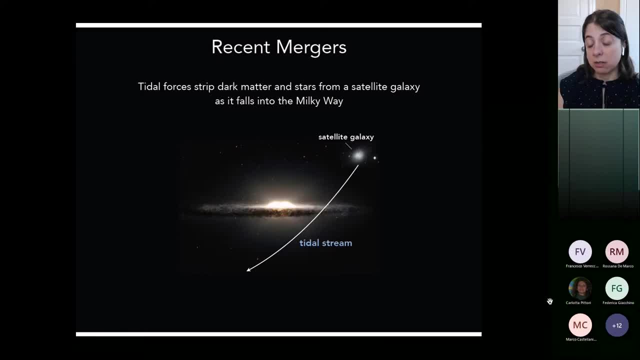 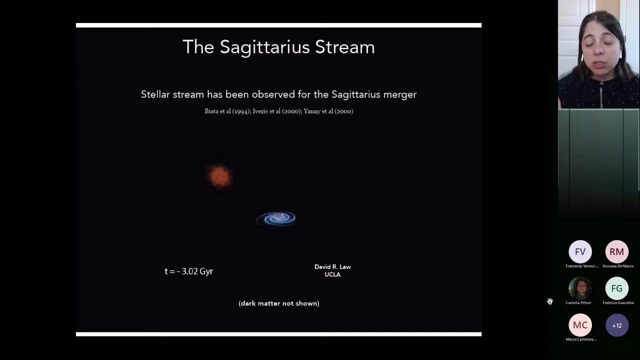 um, both spatially and then also, uh, in velocity. so spatially it really looks like a narrow stream, and if you look at the stars and the dark matter in that stream, they're fairly coherent. um, next slide, um. a large number of these stellar streams have actually been observed in the milky way, which has 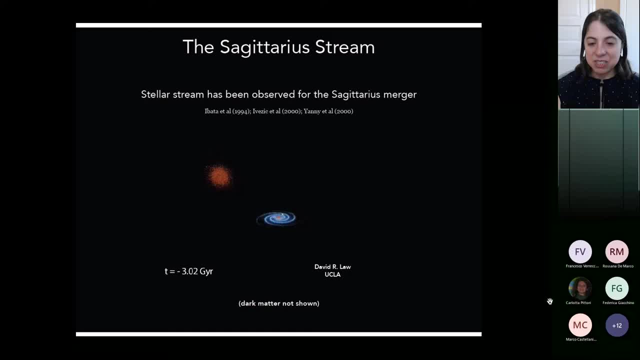 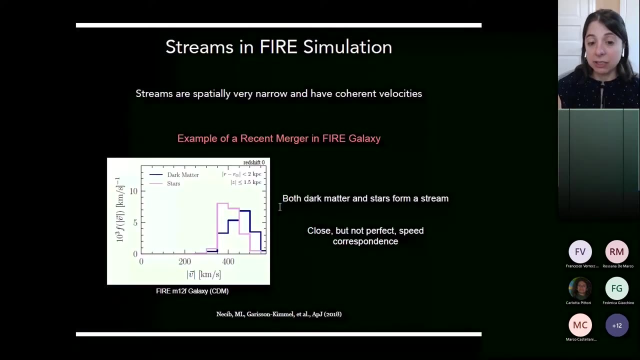 been a uh. it's a beautiful sort of uh representation of you know this process all at work um, and this movie uh would have shown you um the stellar stream that forms uh from the merger of the sagittarius galaxy which is happening uh currently. so sagittarius is actually in the process of being. 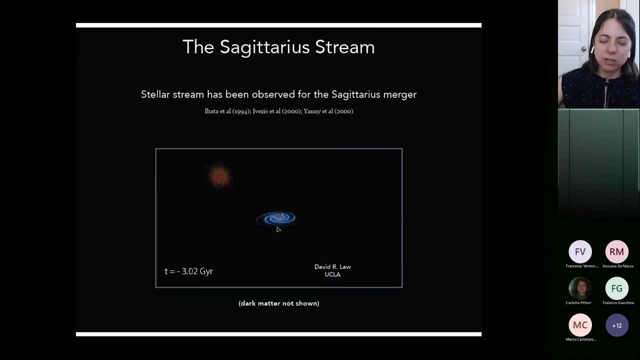 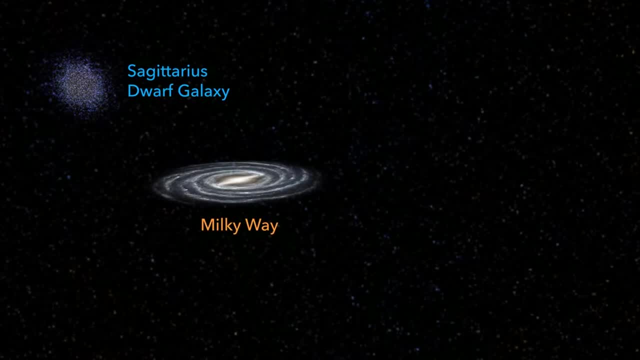 disrupted. and, um, we see a star that's falling in the milky way, and that star is actually a star that's falling in the milky way, and that star is actually track trace out the orbital path of sagittarius. so so, so, so, so so. 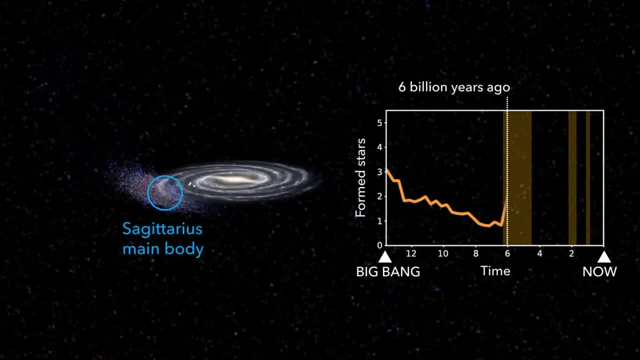 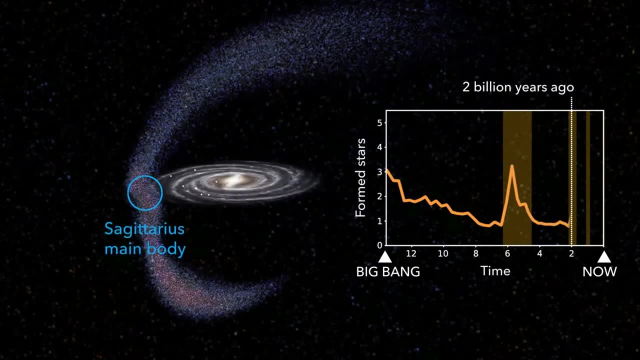 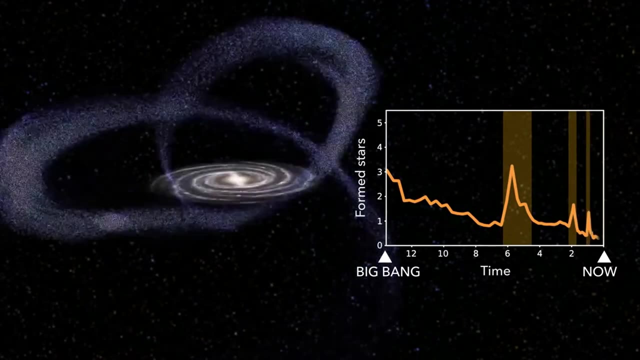 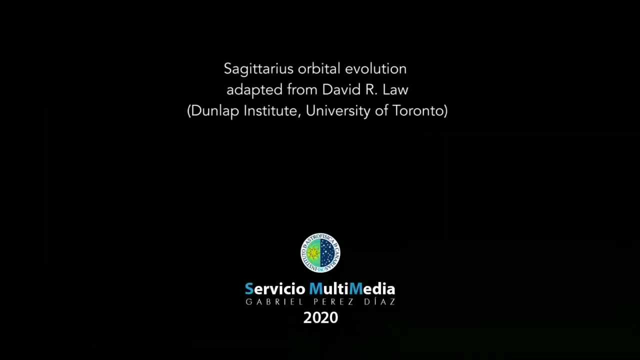 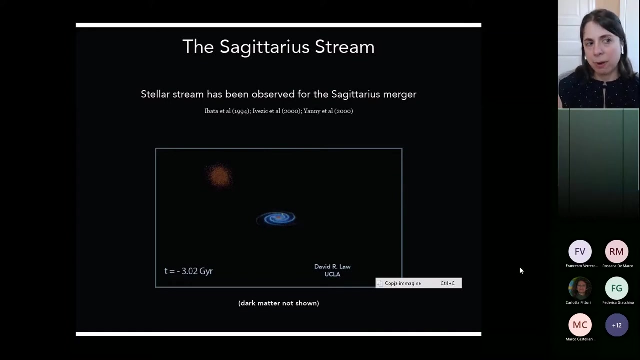 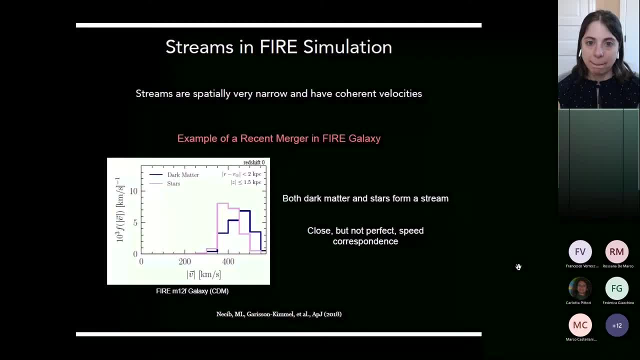 um next slide. uh, so in the fire simulation, um, we can actually go in and identify uh um subpar. uh, so in the fire simulation, um, we can actually go in and identify uh um subpar, um substructure that's removed, that actually looks like stellar streams so we can identify. 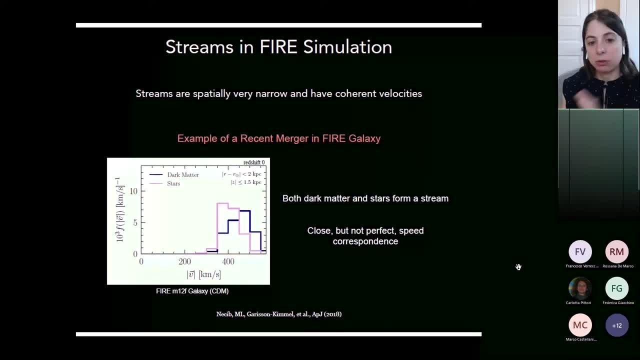 stellar streams and then look to see whether or not there's a corresponding dark matter stream that's coming from the same galaxy and so we can compare. does the dark matter stream really track where the stellar stream is? do they have the same velocities and so forth, and what? 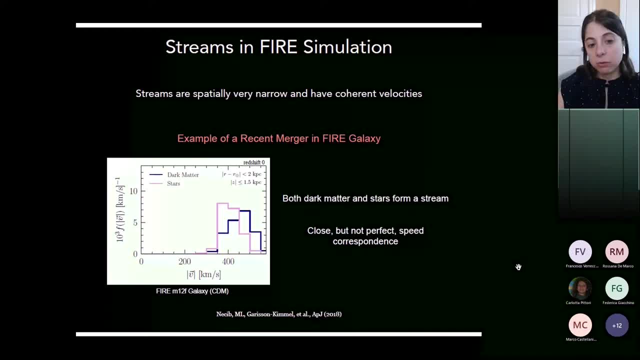 we learned from this exercise is that, in general, if you do form a stellar stream, very often you also have a corresponding dark matter stream, but the two aren't always necessarily directly aligned with each other and, moreover, there could be small differences in their speed distributions. so this is illustrated for a particular example on this plot here, which is just showing a 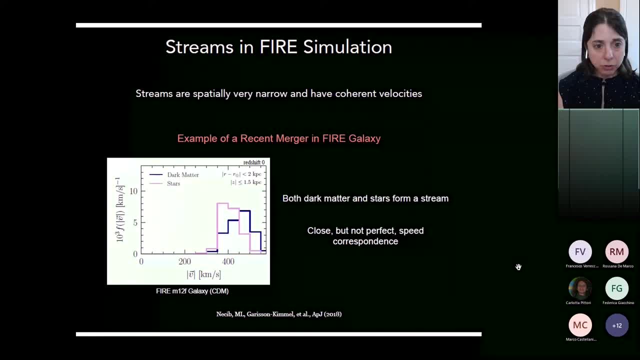 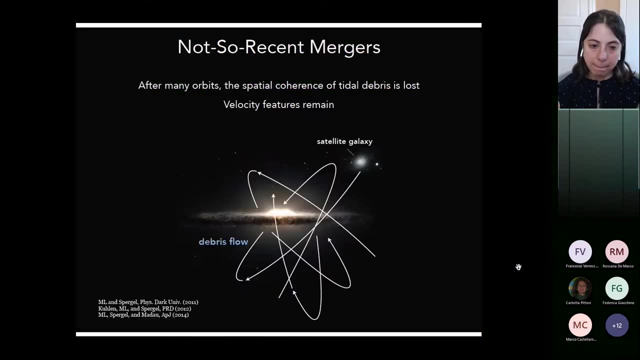 distribution in speeds for a stellar stream that's in pink and its corresponding dark matter stream in blue. so the the velocities in both streams are similar to each other but they aren't in direct uh correspondence uh next slide. so if we continue now with uh sort of moving forward in the evolution of this, 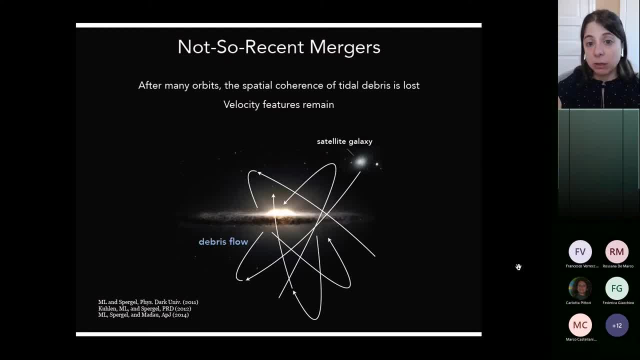 merger. um once that satellite galaxy makes many orbits. um, all of these streams are essentially getting wound up, and you can think of this almost as sort of like winding up a ball of yarn. um, after a certain point you sort of lose the coherence of any individual stream and you just 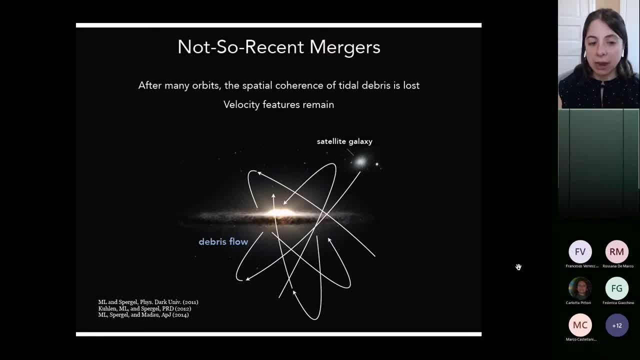 sort of see the material that's gotten removed as kind of a big fluffy cloud of stuff. so spatially everything gets mixed. but what's interesting is that in velocity space that cloud of stuff actually ends up having, um, very distinctive and in some cases, uh, coherent features in the velocity. 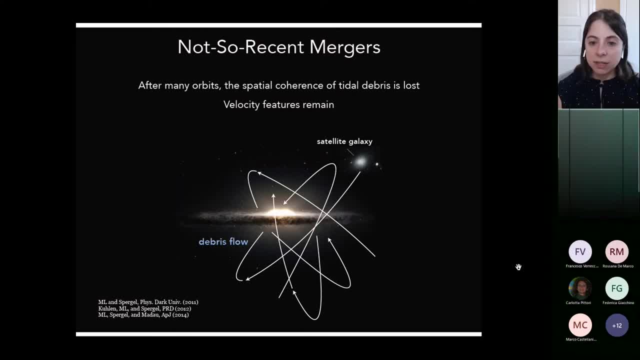 distribution of the material. and that's important because it means that, even though spatially like there's nothing interesting going on, we can actually look for, um, you know, distinctive velocity behavior, to identify, uh, the fact that this material got left behind by a satellite galaxy. um, next slide. 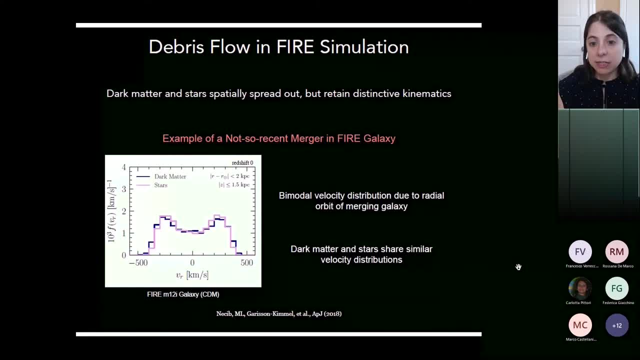 um. so again, if we go into the fire simulation and identify a merger um that sort of came in not so recently, so one that essentially had an opportunity to make many of these orbital passes, and then we can look at the- both the stellar material and dark matter material that it left, 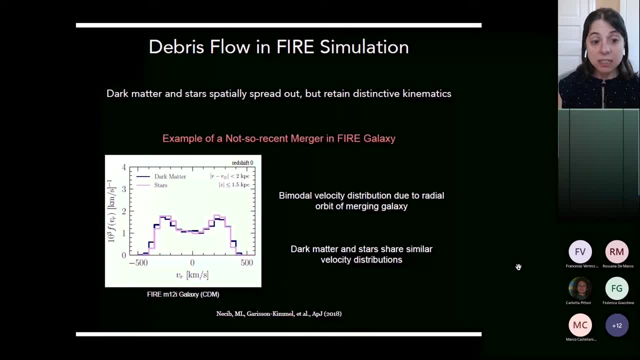 um, what we find in this case is that indeed, uh, both the stars in the dark matter sort of spatially, don't really? they look sort of like fluffy clouds. there's nothing interesting going on there, but when we zoom in and we look at their velocity behavior, oftentimes you end up seeing like 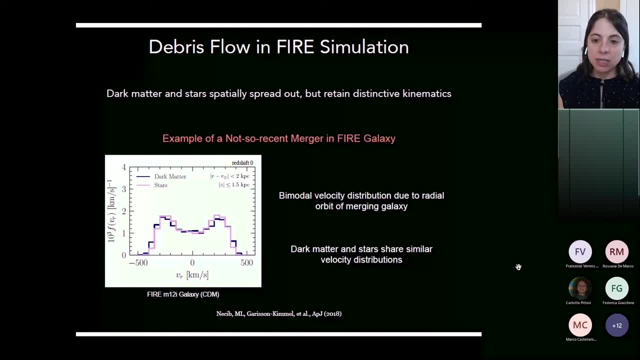 bimodal distributions, interesting shapes there that are reflective of the orbital properties of that merging galaxy and, moreover, for these particular instances, because the material is more well mixed, both the dark matter and the stellar velocity distributions track each other really well, um. so this is interesting and really heartening because it 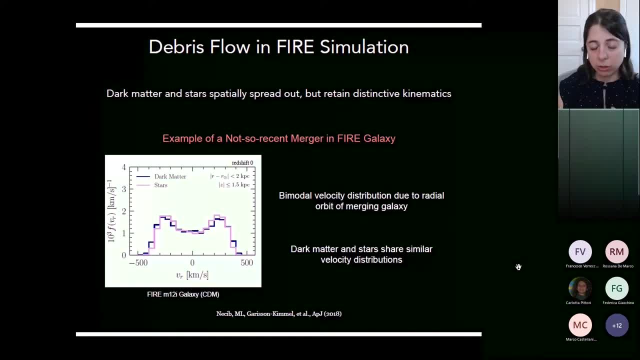 suggests that if we do find evidence for one of these older mergers in the gaia data that the velocity distribution of the stars that would have originated from that merger, um would, would track nicely and be a good indicator for the dark matter that would have also gotten left behind by 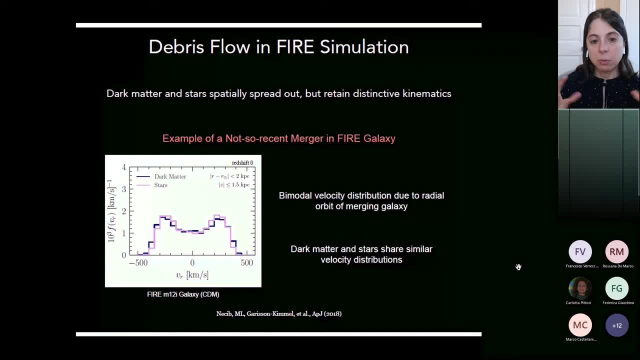 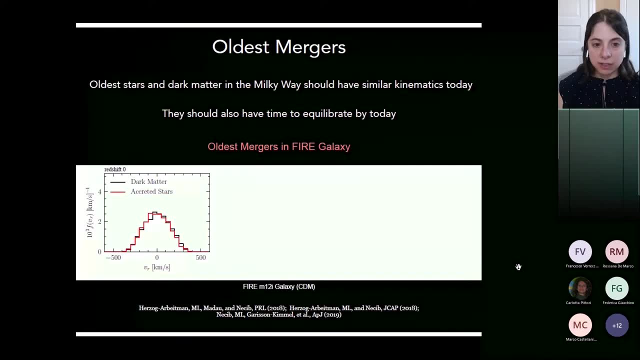 that merger. um and again, all of the statements that i'm making here are specific to the solar neighborhood. next slide. so the the last stage of this evolution is mergers that came in very, very, uh, early on. and so this is. these are mergers that have left behind stars and dark matter in the 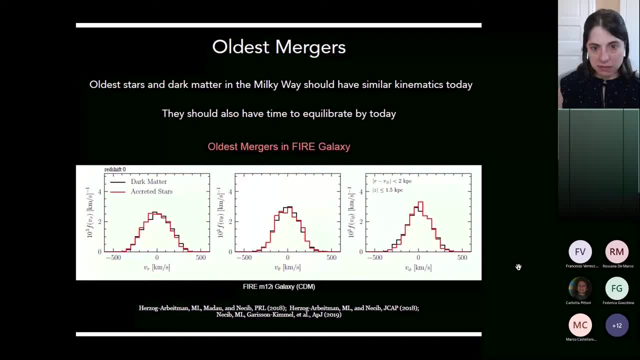 milky way and the stars and dark matter have had tons of time essentially to uh, come into equilibrium and to, to, to virilize by the present day. and so if we go into the fire simulations and we look at only these very old mergers- and these are typically galaxies that came in um before redshift of three- 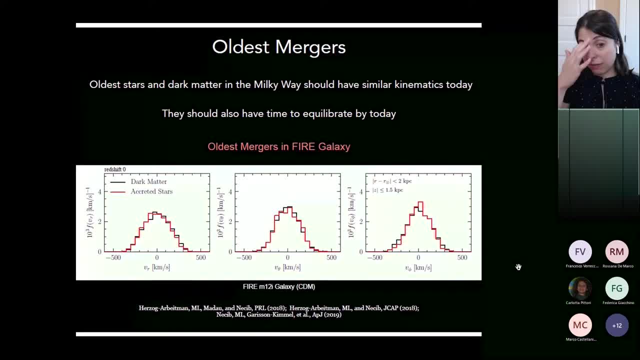 or so, and we look to see what, how their dark matter and stars are behaving today. what we find is that, um, the velocity distribution is usually isotropic. it does look sort of maxwell boltzmini um and that the dark matter and the stars from these really old mergers are going to be 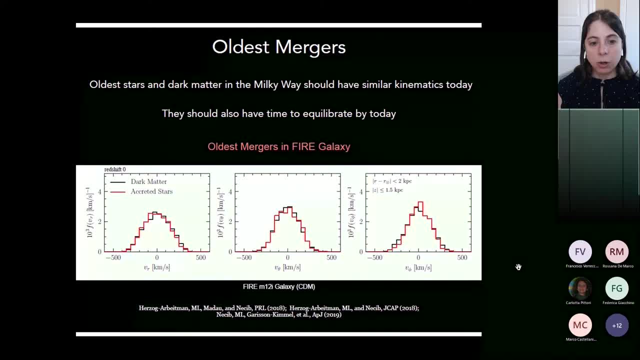 almost perfectly. so, um, uh, yeah. so this allows us then to also uh. this also suggests that the accreted stars can serve as a good tracer for some of the- uh, dark matter that would have come from these oldest mergers. next slide: um, okay, so this is just a summary now of how we've been thinking. 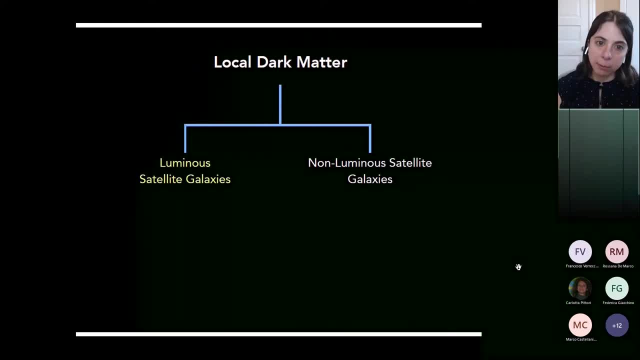 of uh sort of the process by which you would sort of create a map of the dark matter near the solar position, um, with an understanding of what the merger history of the galaxy is. uh. so the ultimate goal right is to create that map, and the way we're thinking of doing that is essentially by 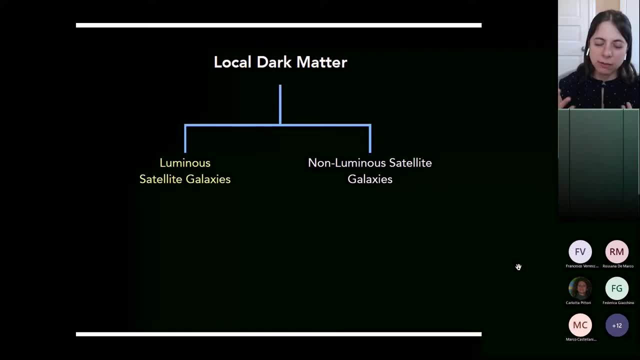 understanding which satellite galaxies would have contributed material near the solar position. of those satellite galaxies, we're dividing them in two separate categories, so the ones that are large enough to actually be luminous and have enough stars in them, and then the ones that are less massive and don't have any stars, and then the ones that are less massive and don't have any stars. 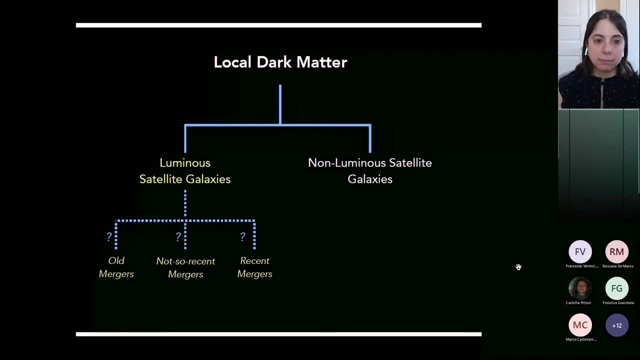 in them. so these would be like dark galaxies, um and uh. where we've been, you know, making the most progress to date is essentially on the arm of this diagram for the luminous satellite galaxies. so that's the arm where we can use the stars that would have also been removed from those galaxies. 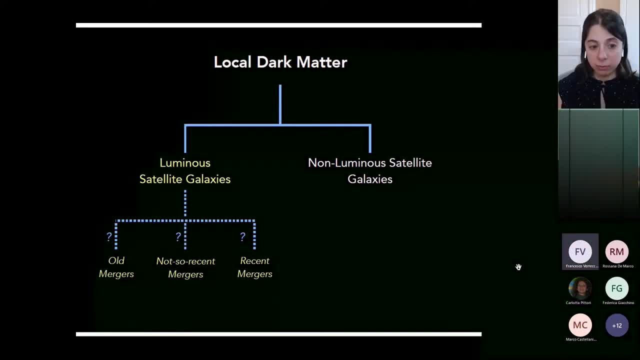 to learn something about the underlying dark matter that would have come from those galaxies, and so we can use these stellar tracers to identify these mergers, whether or not the mergers were very old, not so recent or came in very recently. and then, based off of that, 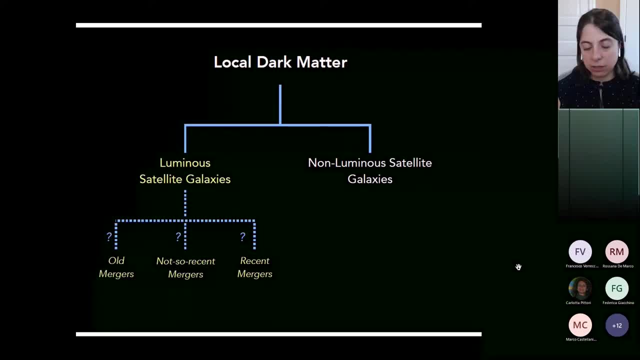 um, uh, understand what the underlying like, how the underlying dark matter distribution should be behaving. um so, uh, you know, maybe like five or so years ago, we really had no understanding of how to do this mapping of the local dark matter. and i think, with the advent of gaia and also combining all of that, 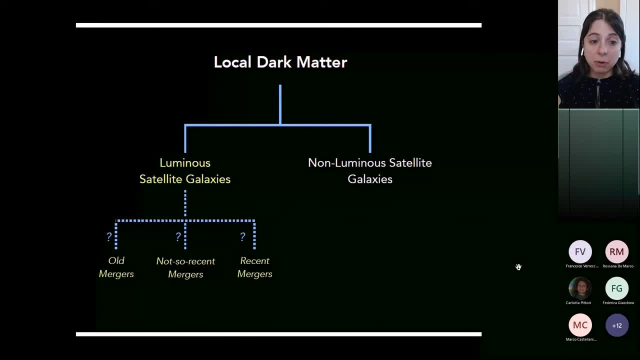 with what we've been learning from simulations, we've been able to make a lot of progress on understanding that local dark matter distribution in the galaxy um and in the solar system as a whole. there's nothing that we can do that could help us in principle to. in my opinion. I think that's the image of a new. we could've used the data. that would be, we could have used a lot of data. we could have used the data, but that wouldn't have been enough information to know, would it not? 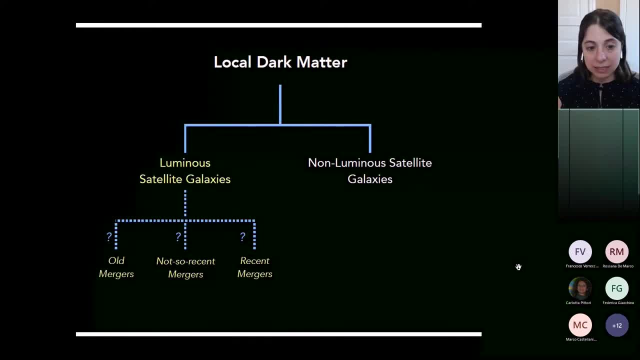 local dark matter piece from coming from the luminous satellite galaxies Where we haven't quite dug in yet. but this is definitely future work is understanding how to also build up the component that's coming from the dark galaxies. But for the rest of the talk I'm going to really 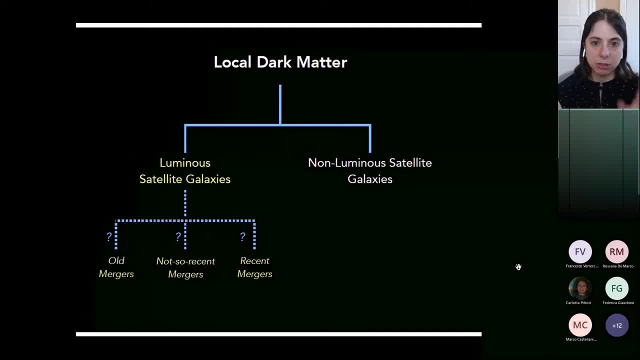 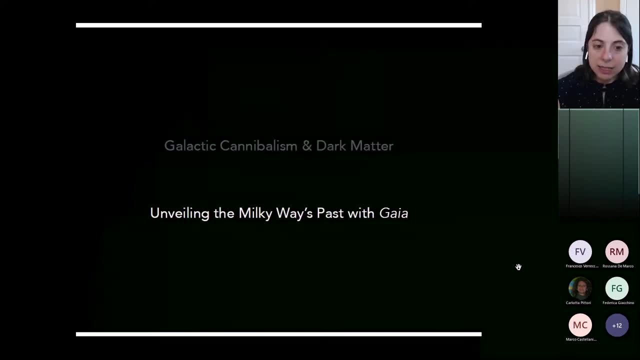 be focusing on the advancements we've made from coming from the dark matter that originated from these luminous satellites. Next slide: Okay, so that leads me to the second part of the talk. focusing on this is going to be more focused on actually the Gaia data and what we've been. 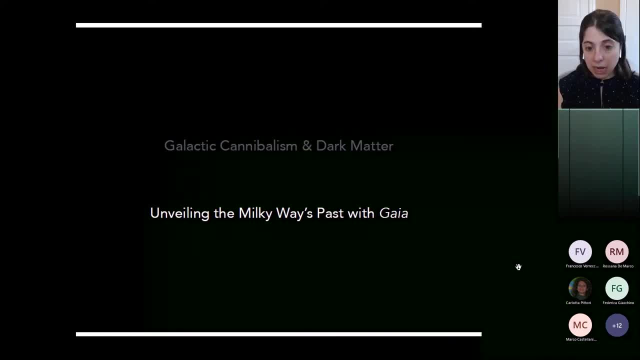 learning about the Milky Way's historical evolution and how we tie that in to the local dark matter distribution. Next slide. So Gaia is the follow-up astrometric survey to Hipparcos, which is a very important data source for the Milky Way, And it's a very important data source. 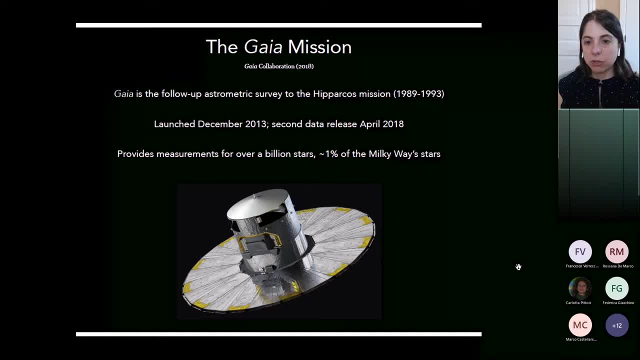 for the Milky Way And it's a very important data source for the Milky Way And it's a very important which ran in the early 1990s. It was launched in December 2013.. The second data release was a few years ago And the community is ramping up and getting really excited because the third data 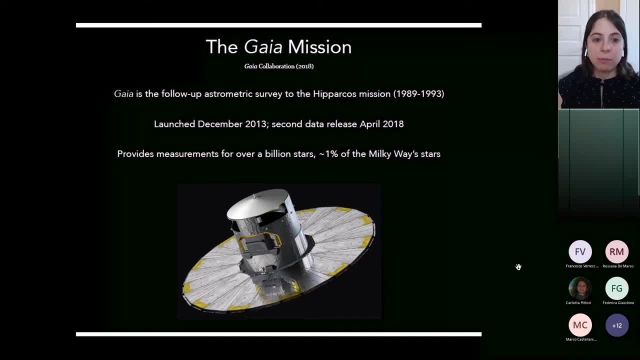 release is coming this June. The advancement from Gaia that Gaia has made from Hipparcos is tremendous. It provides measurements for over a billion stars in the galaxy, which is about 1% of the Milky Way stars. It's far more than we've ever. 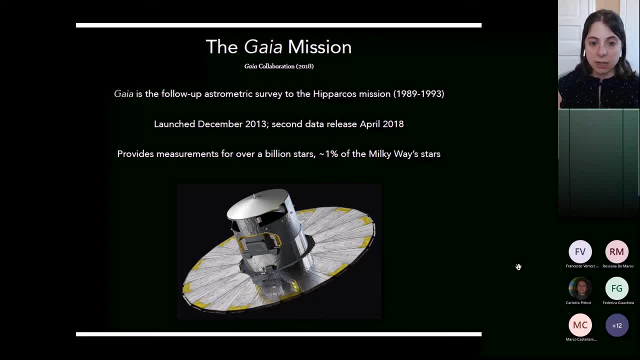 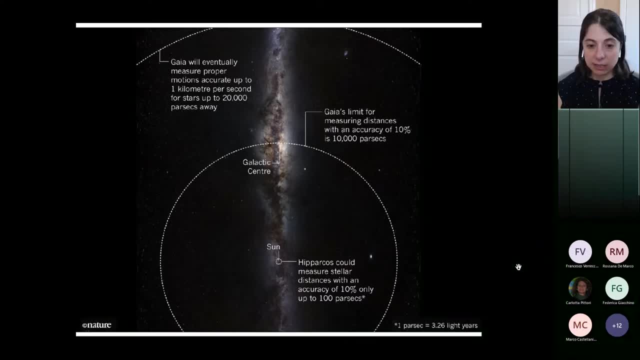 been able to sample Next slide And just to kind of give you a quick sense for that sort of scale of the difference. this is the Milky Way galaxy, but rotated up, So going vertical is the disk and the sun is in the bottom, The little dotted line, dotted circle. 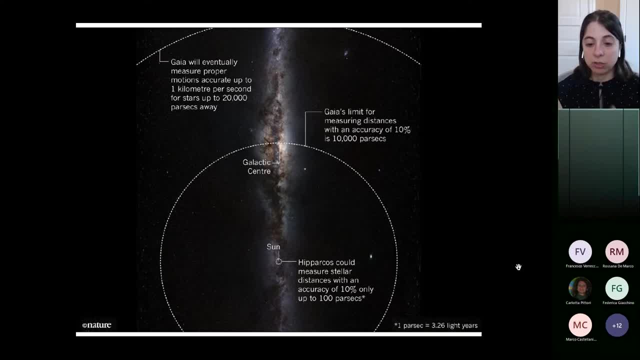 around the sun is the region where Hipparcos was able to measure stellar distances with an accuracy of 10%, And the core of the circle is the Milky Way. And the core of the circle is the Milky Way. The corresponding region where Gaia has that same level of precision is shown by the next outer. 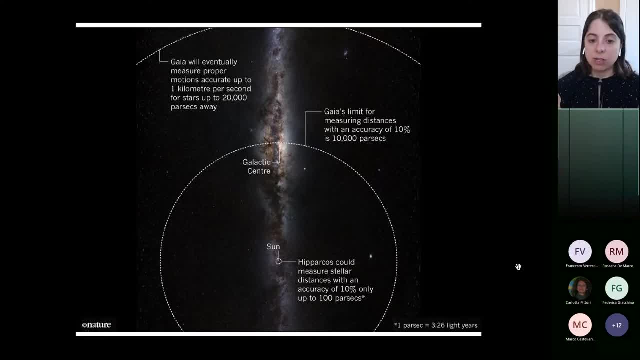 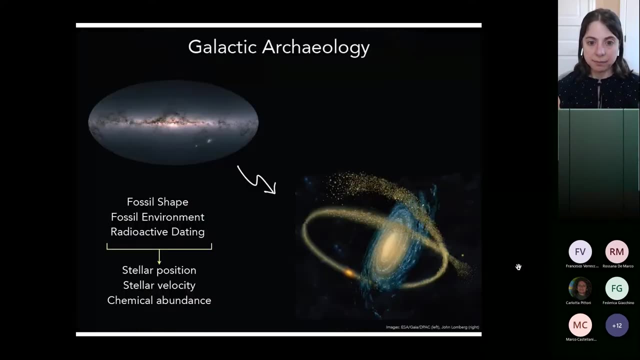 circle. So with Gaia we can get this mapping that goes out much, much further. So it's a spectacular opportunity to be able to look for material that would have gotten left behind by these satellites Next slide. So what is actually the plot Like? how does one do this? It's challenging. 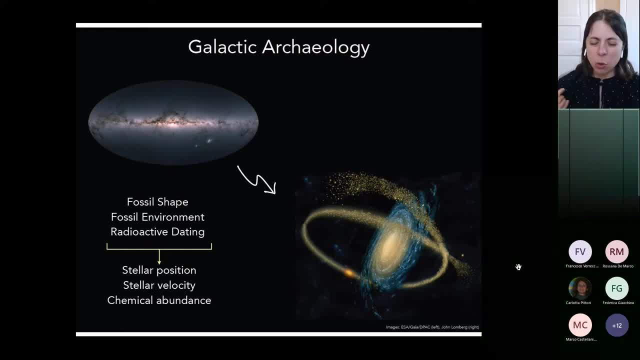 to find the stars in the Gaia data are actually stars that were born in the Milky Way and are forming the Milky Way's stellar disk. So in trying to find stars that would have come from a merging galaxy, it's really a it's a rare event search, essentially, And so in order to do this effectively, 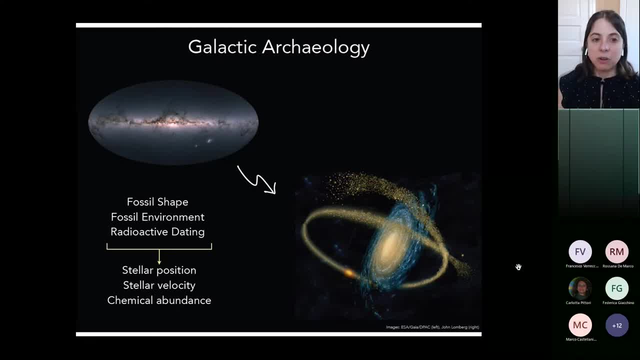 it's a bit like going on an archaeological dig. So on an archaeological dig you might find a fossil and then you would use something about it to find the stars, And so it's a bit like going on an archaeological dig. So on an archaeological dig you might use something about the shape of 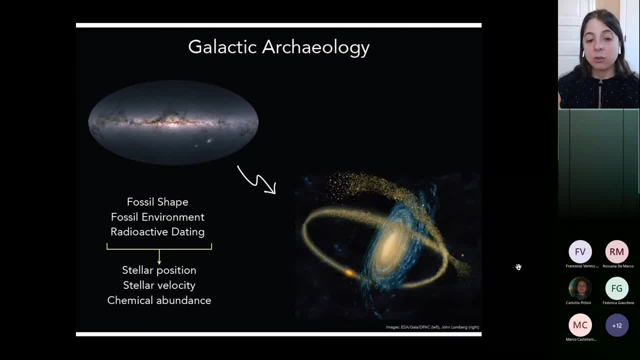 the fossil, maybe its environment? maybe you might do some radioactive dating to try to figure out the creature that it came from and when that feature might have lived. In a similar way, we can go into the Gaia data and use information about stellar positions, their velocities and perhaps 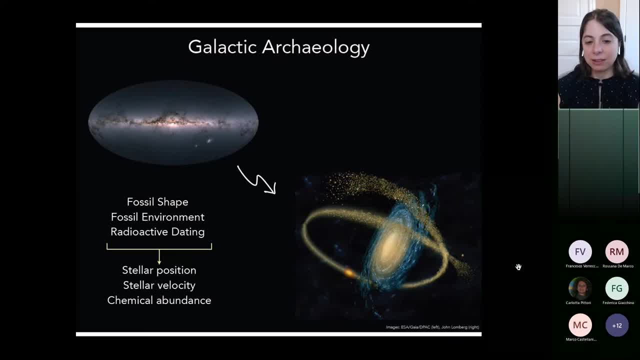 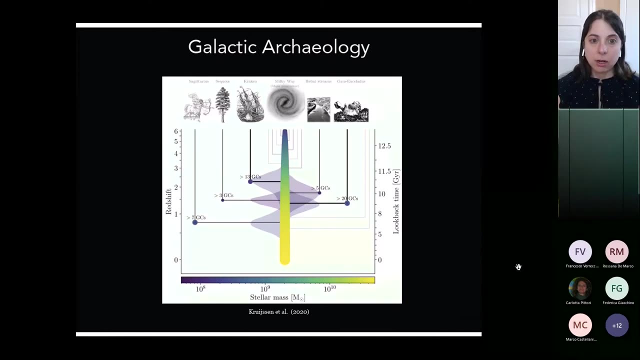 their chemical abundance, to try to infer the sort of satellite, the galaxy from which it came and to infer the sort of full picture of the evolution of that satellite galaxy Next slide. There's been a vast effort on this over the last few years And the you know the galaxies that 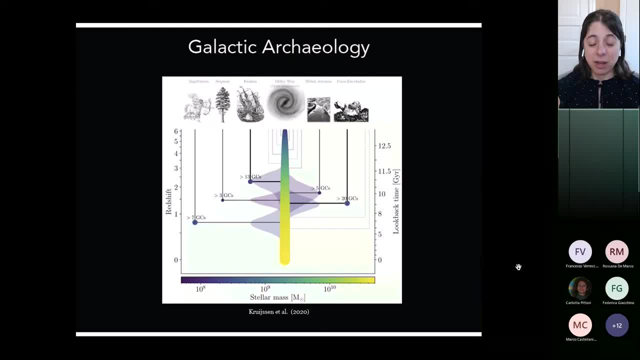 you know, a variety of these galaxies have been mergers, have been hypothesized and based off of the data. This is just a really sort of- I think it's a sort of very nice way of illustrating this, so I thought I'd include this. So this is kind of a mapping going back in time, So present day. 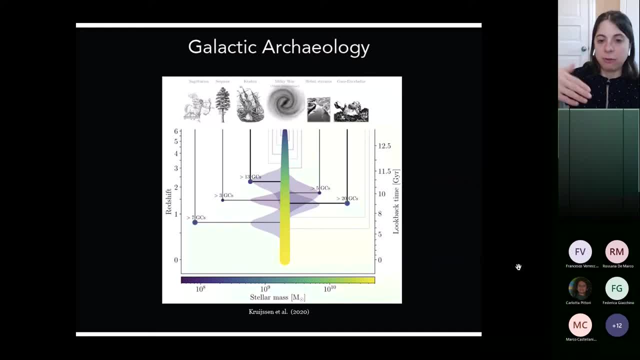 would be at the bottom. And then, as you go into the further, into the past of the Milky Way, that's, you're moving up And the arrows, the black lines, are indicating tying points when we think that one of these mergers might have happened. So there's the Sagittarius galaxy, which I mentioned earlier. 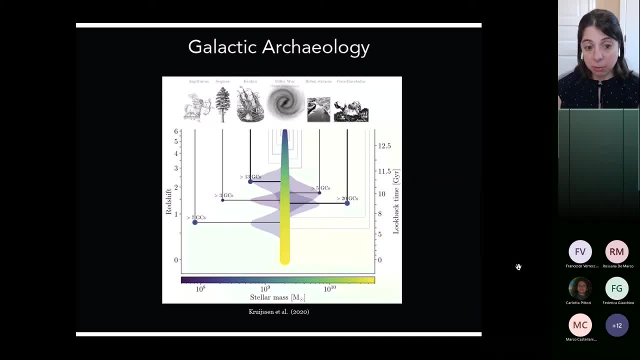 that we actually see in the process of falling in and being disrupted. You know that likely started that process, you know, maybe like six or so giga years ago, And then, as you work backwards, there's other galaxies that are moving up and you're moving up And the arrows, the black lines are indicating. 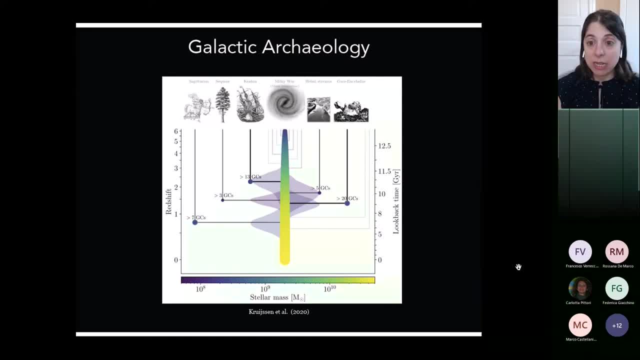 these galaxies that have been other merging events that have been identified. Another one that I'll spend quite a bit talk quite a bit talking about later is this Gaia and Solatus merger, which is hypothesized to have occurred sometime between eight to ten giga years ago. Next slide: 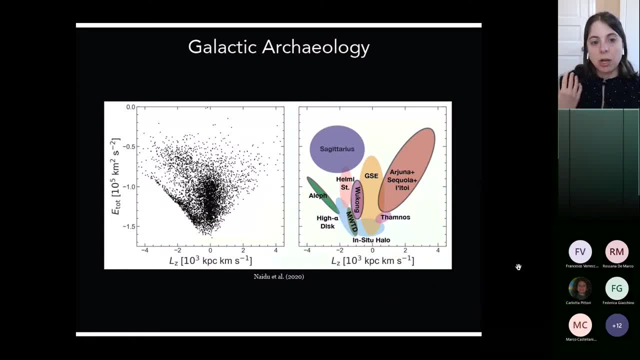 This is another way of kind of looking at the same picture. So the way people identify that these mergers occurred is by looking for patterns in the kinematics or energy and angular momentum distribution of the stars. So this is work from the H3 survey And on the left panel you see total energy as a function. 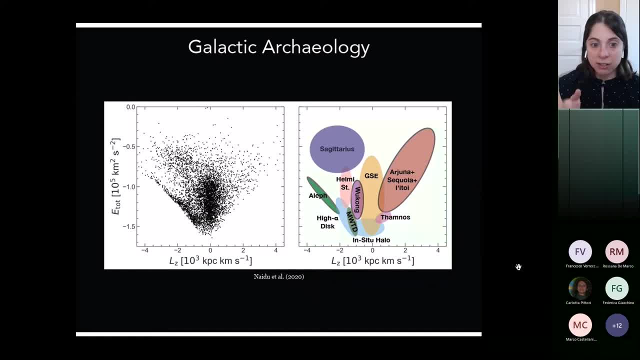 of angular momentum in the z-direction. Each dot represents a star in this space And you know it sort of looks like a big blob of stuff but there's actually a lot of structure that's there And all of the work sort of goes into figuring out how to actually divide that up. 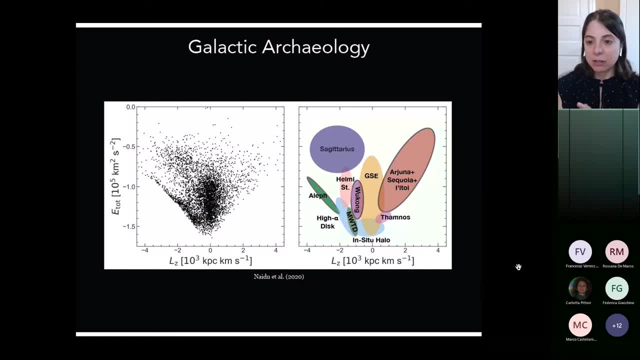 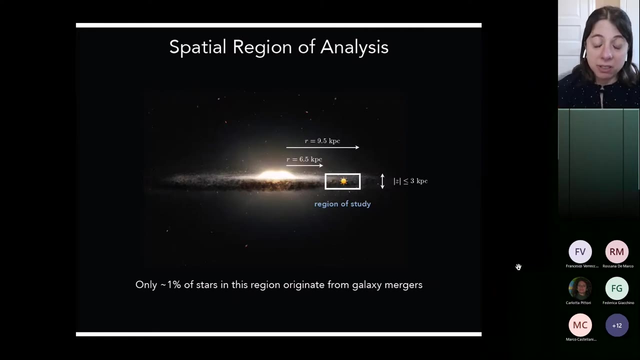 into, you know, structures that make sense, And on the right is a very sort of illustrative mapping of where particular clusters are thought to be, And in some case those clusters might be associated with a particular satellite merger Next slide. So our goal for the sort of rest of the talk is to essentially go through this. 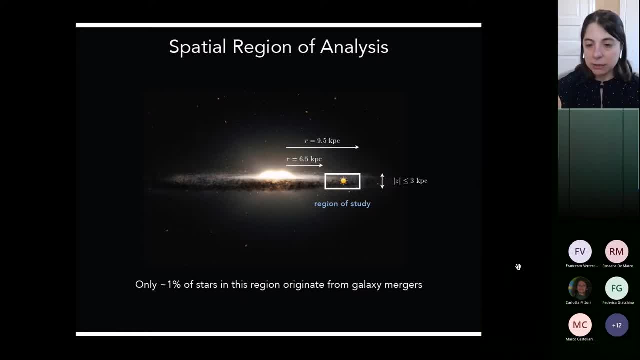 exercise, but focusing really on the region around where the sun is So, which I've indicated here by this white box. this is a particularly difficult region to do this exercise in, because you have a huge amount of contamination from stars that were born in situ. 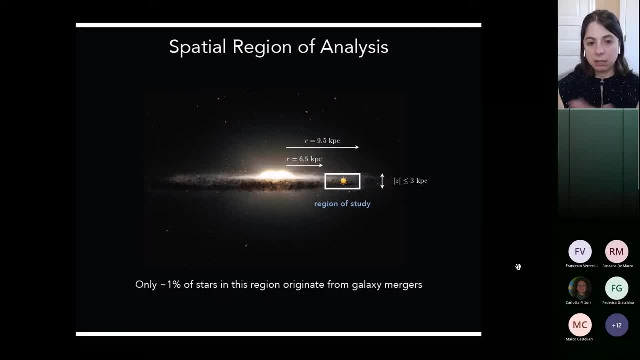 or that's just another way of saying that they were born in the Milky Way, in the, in its stellar disk. So you, essentially, you have to be able to sift through all of that in order to be able to identify the- you know, maybe 1% of those stars that might have originated. 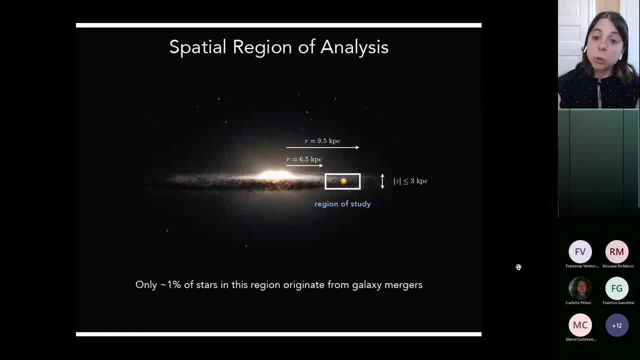 from the galaxy merger. But this is essentially the effort that we need to go through if we want to really understand what satellite mergers dumped things near the sun, Because if we can map that out from the stars, we can then try to infer what that would have done to the dark matter near the. 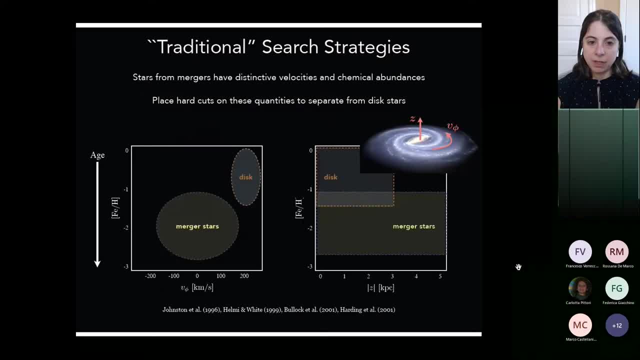 sun Next slide. So a very traditional way of doing these kinds of searches is to try to figure out how to separate out the stars from the sun, And so what we're going to do is we're going to look at the stars that would have been born in the Milky Way's disk from those that would have 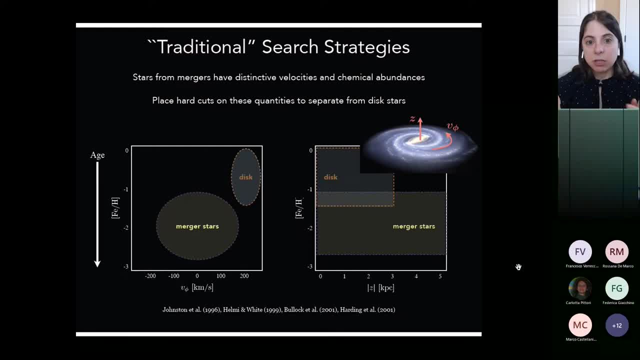 come in from a merger by sort of slicing in particular regions of parameter space where you think that the disk stars should be separated from the merger stars. So this is very illustrative but it's just a little cartoon thing, but just to kind of show how this would work in particular. 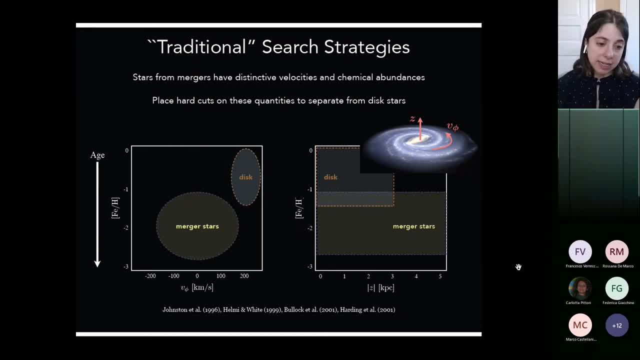 along particular parameters. So on the left is a plot, little schematic plot, of circular velocity of the stars. So this would be their orbital velocity around the center of the galaxy, And vertical axis is their metallicity, which you can think of as epoxy for the age of the stars. 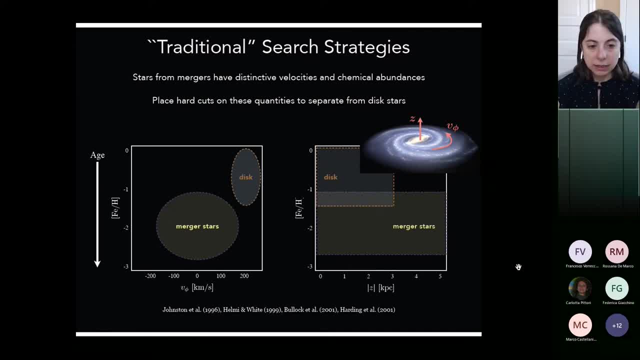 with the age increasing as you go down the y-axis. So the stars that were born in the Milky Way would sort of cluster up in the top right of that, where the ages of the stars would be pretty young, and then they would all be sort of rotating around with roughly 200. 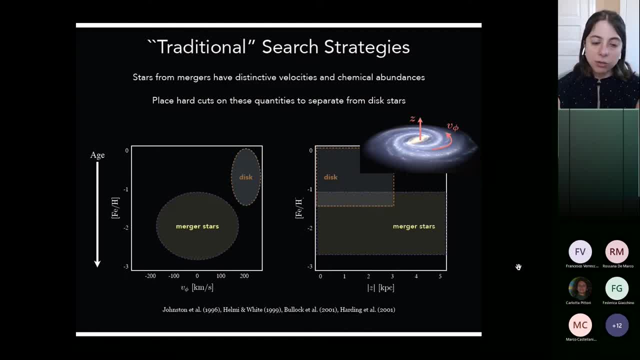 kilometers, a second circular velocity, And stars from mergers don't necessarily follow this pattern. They'll typically be older, so they'll fall lower in and down on this plane and their velocities might have more of a spread. They may not necessarily be moving around with 200. 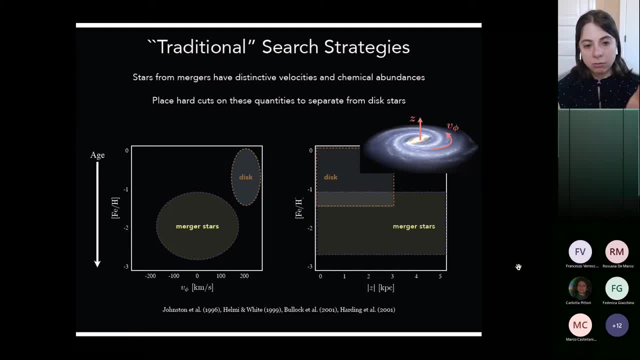 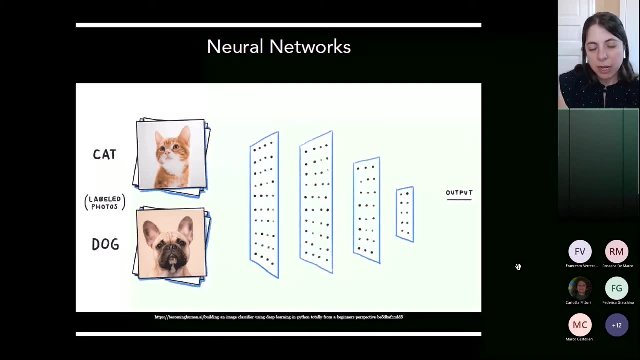 kilometers a second. So one way to you know sort of slice out the disk stars is to just put a cut and remove everything that's you know from the right top region of the plot Next slide. Our approach, for the results I'm going to show you next, is a bit different. 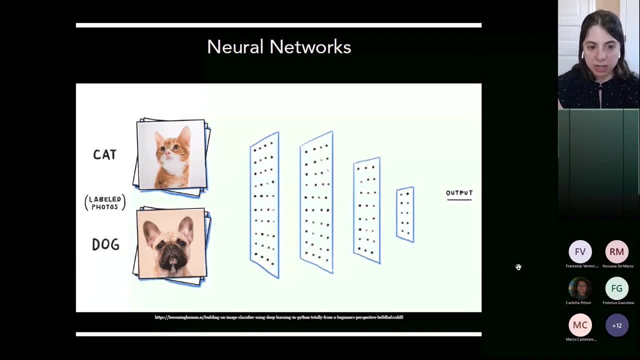 What we wanted to be able to do was to see if we could train a neural network to better distinguish stars that would have been born in situ- sort of disk stars- from those that would have come from these merging satellite galaxies. This is a classification problem, and what this was- a little animated movie just showing. 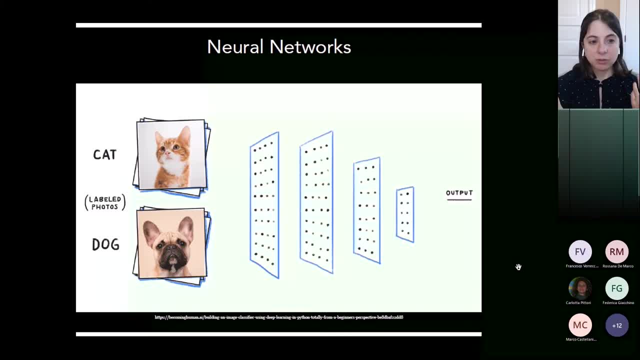 cartoon of a neural network And when you train it on a bunch of labeled photographs of cats and dogs and you know, the network then ends up learn, learning how to classify photos that look like a cat and photos that look like a dog. Next slide. 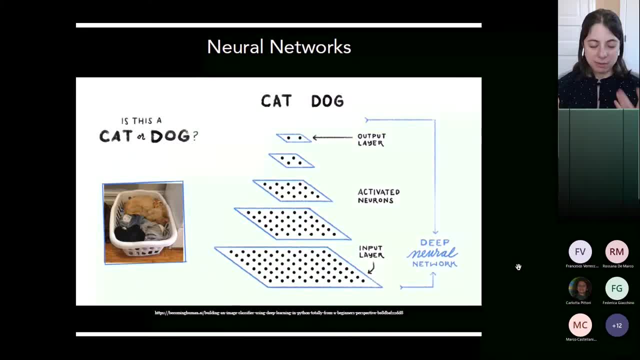 And so you go through that training process using a set of labeled photos And then, once the training process is done, then you can give your neural network a random photo like this one and then have it take its own. You can then give it a random photo and then have it take its own. 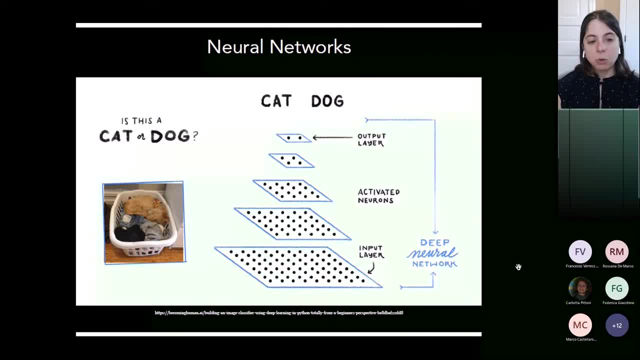 best guess as to whether or not that's a cat or a dog. So our setup is sort of similar to this, except instead of training the neural network on cats or dogs, we're training it on samples of stars that would be known to be born outside of the Milky Way, in some satellite galaxy versus. 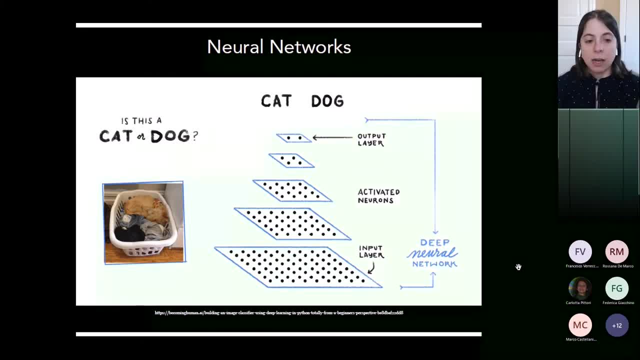 stars that would be born in the Milky Way disk. The only reason that we have a shot at being able to actually do this is that we actually have good training sets, because simulations have actually been getting a lot better at reproducing galaxies that look similar to the Milky Way. 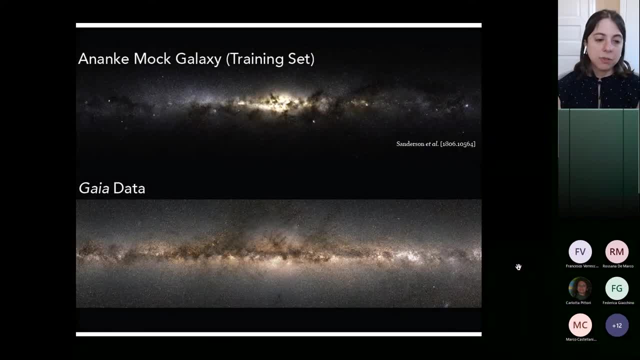 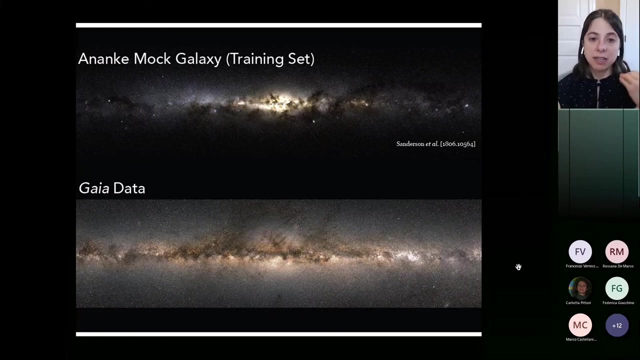 Next slide. So this is a result essentially illustrating this. So on the bottom is the actual data from Gaia and on the top is a mock galaxy That's generated from simulation. So it's essentially given some simulation of a Milky Way-like galaxy. a mock Gaia data set is generated from that. It looks like the top panel. 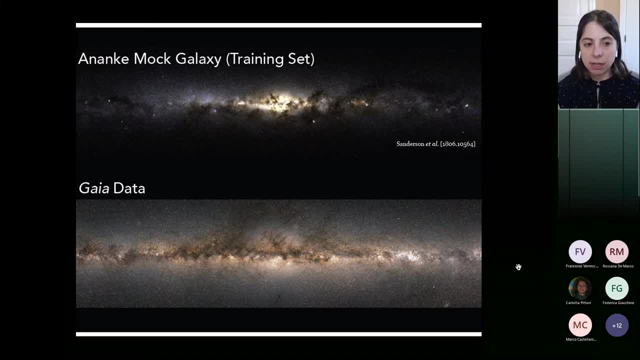 And you can see that there's a lot of features that are similar between the mock galaxy and the real data. In particular, you're forming a stable disk. There's a lot of structure. You see areas where there's gas that's obscuring the light, other regions where you actually get a lot more. 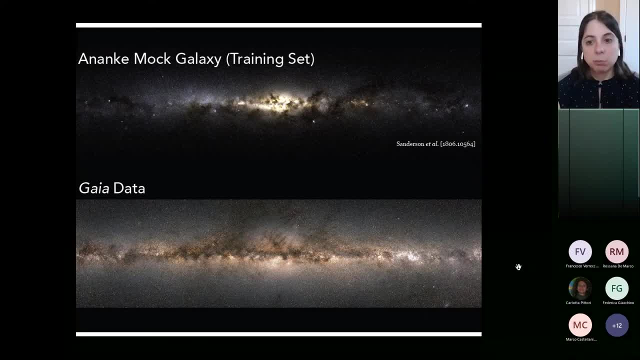 light that's coming through. Reproduction isn't exact by any means, but it's pretty close, And that at least gives us hope that if we were to use these mock galaxies as a training set to build a network that can identify accreted stars, we might actually have a shot at being able to do this in the real data. Next slide: 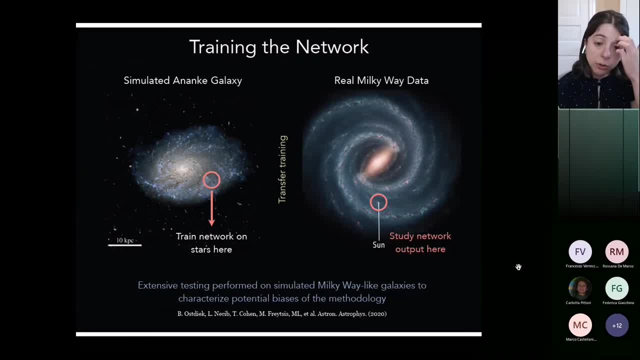 So this is the procedure we used for training the network. We start with a simulation of a galaxy that looks like a real galaxy, And then we have a simulated Ananka galaxy. We train the network on stars in one part of that galaxy, And then we 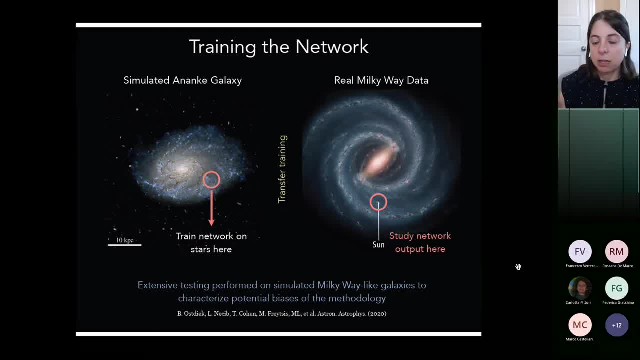 essentially apply it to the real Milky Way data under the solar position And the network at that point, because of its training, is essentially going to spit out a prediction for each star and with essentially a probability of whether or not that star was born in the Milky Way disk or 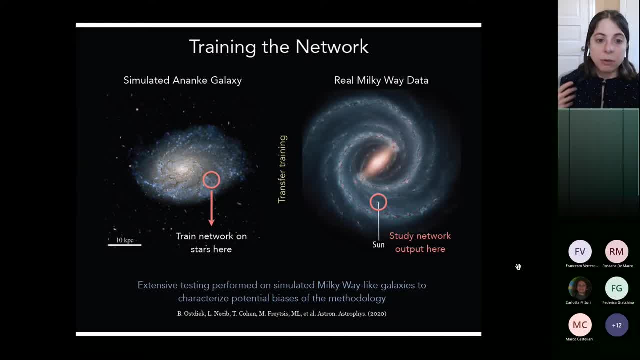 whether or not it came in from the Milky Way disk, And then we apply it to the real Milky Way data. Now there's a lot of ways that this kind of procedure could go wrong, And when we first started working on this, I actually just didn't think it was going to work. So we went through a 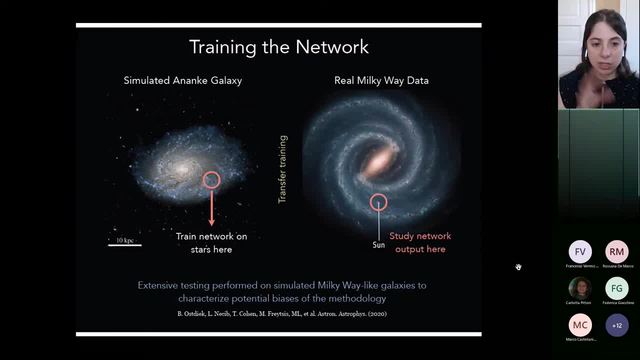 very long process of over a year of essentially testing this on simulated Milky Way-like galaxies, to make sure that we understood the biases in this procedure. Just to kind of quickly give you a sense of how we did that. So we started with the simulated galaxy And we essentially trained the network on a subset of stars. 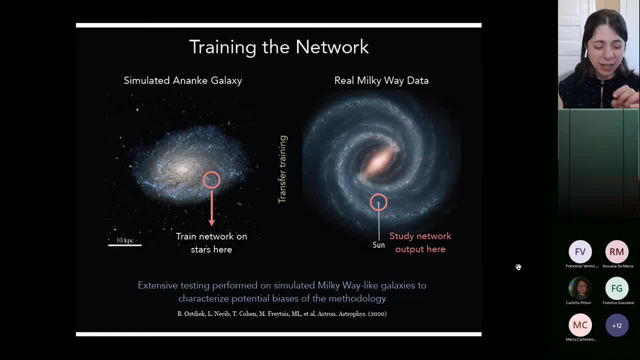 that were near the one particular solar position And then, because we knew the truth information, because it was a simulated galaxy, we could see how well we did at sort of predicting the accreted versus not accreted label in that particular location of the galaxy. 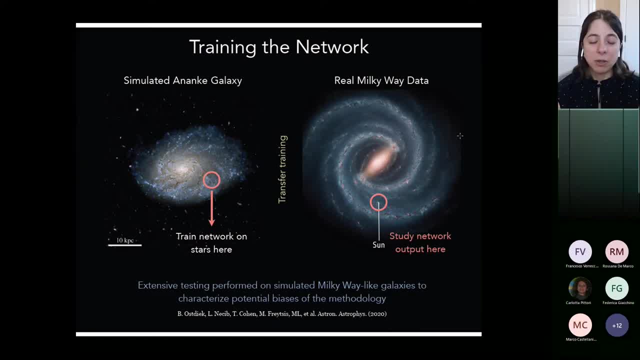 Once that was successful, then what we did was we trained the network on a different part of the simulated galaxy and saw how well it did at predicting the label in a separate. So we sort of the training and the testing set were in a different part of the galaxy. That also worked well. You would still be concerned, though, that the network 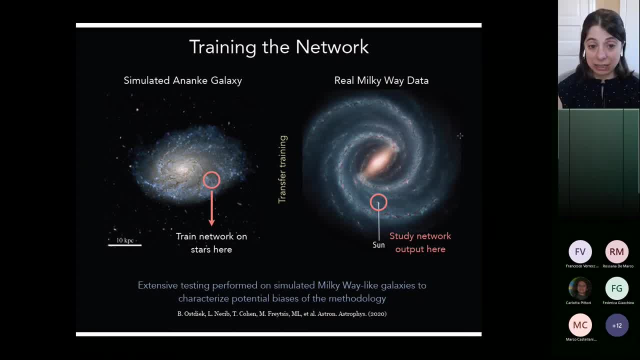 is learning something very specific about the merger history of the simulated galaxy. So, in order to deal with that concern, what we did was we tried training the network on one simulated galaxy and testing it on a very, very different simulated galaxy, And it also worked well in that case, And it was that test that gave us confidence. 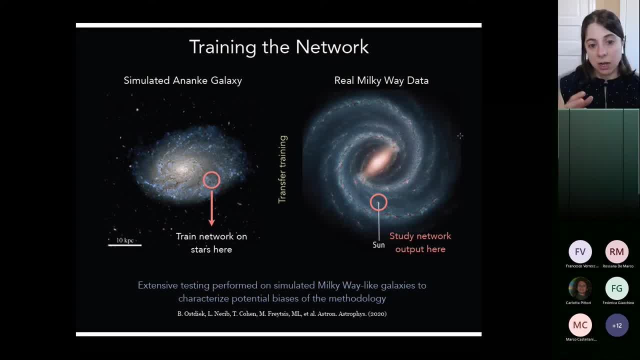 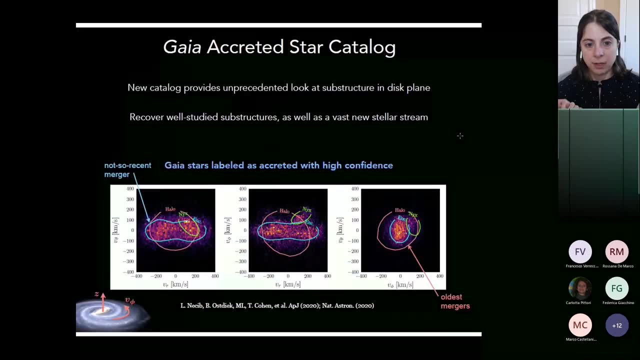 that we would be able to effectively take this and actually use it on the data Next slide. So I'll now just go through and walk you through the results that we got from doing this analysis, because it sort of sheds light on exactly where we are in terms of our 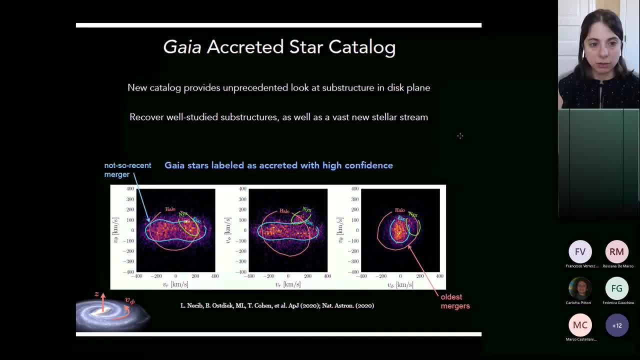 understanding of the local dark matter distribution. So by running the neural network on the Gaia data, what we end up getting is a catalog of all of the local stars that the network predicts with high confidence to have come from another merger satellite, And those stars that the network predicts with high confidence to be accreted are shown. 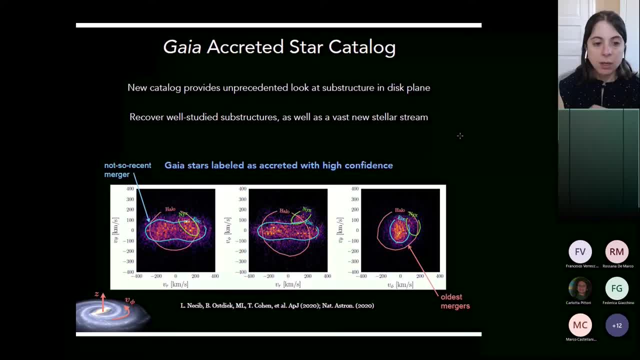 by the density histogram in these three panels here, And there's essentially three separate contributions that are feeding into this, And I'll walk you through this now. So the first contribution is indicated by the pale pink circle and it's labeled halo. Those are, as you can see. 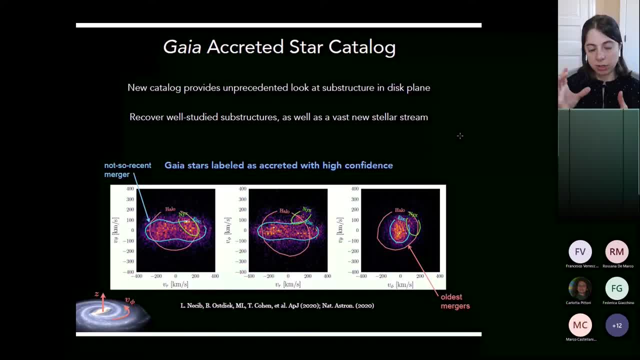 in each of these velocity panels. it's almost a perfect circle. So this would be the stars that would have come in from very, very old, The oldest stars. would have come in from very, very old- The oldest mergers- So they would have had enough time to come into equilibrium and we see them. 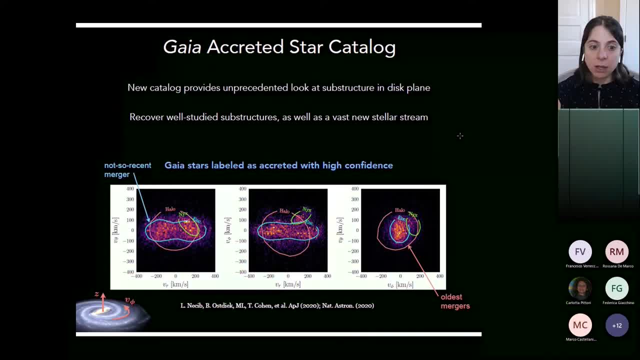 as sort of having this isotropic velocity distribution today. So that tells us that there is some fraction of dark matter near the sun that would have come in from luminous galaxies that merged in before redshift three. So we know that that's a piece of the puzzle. 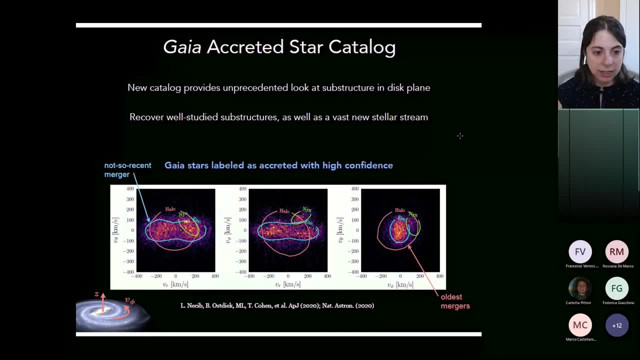 The second component that's important is circled in blue. That's coming from a merger that was identified in the literature. If you go to the next slide, In some papers it's referred to as Gaia sausage. In other papers it's referred to as Gaia Enceladus. 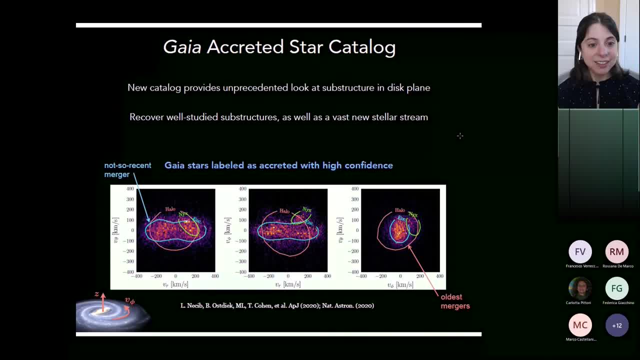 So some other papers refer to it as Gaia sausage Enceladus, so that's what I'll be referring to it as the rest of the talk. so, GSE, The reason it's referred to as a sausage is that because it has a sort of elongated shape in the radial ball, It's a little bit more viscous and it's 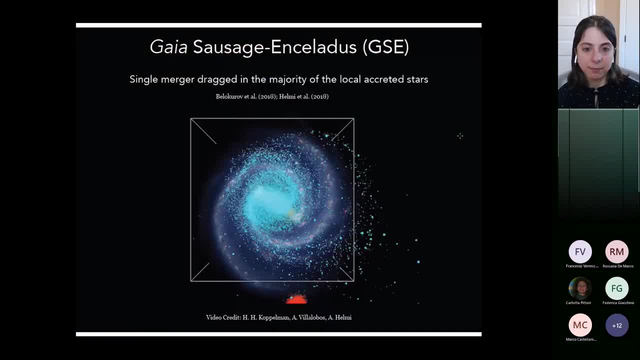 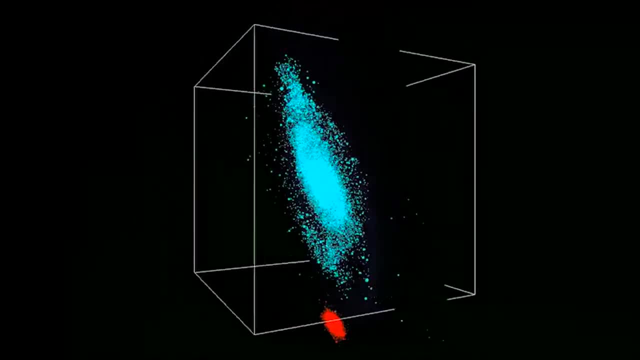 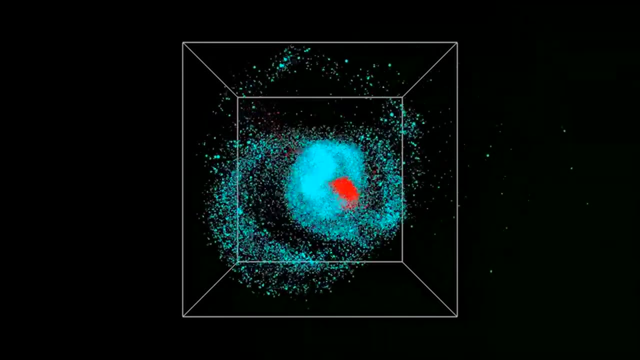 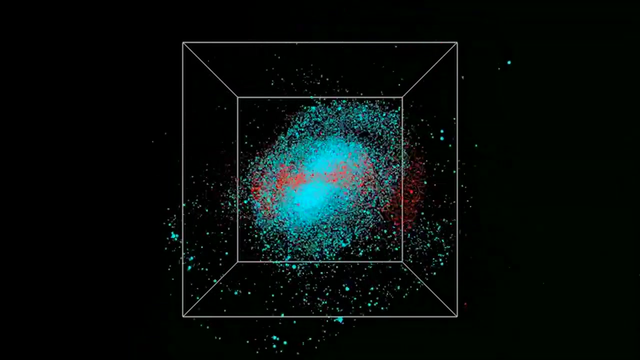 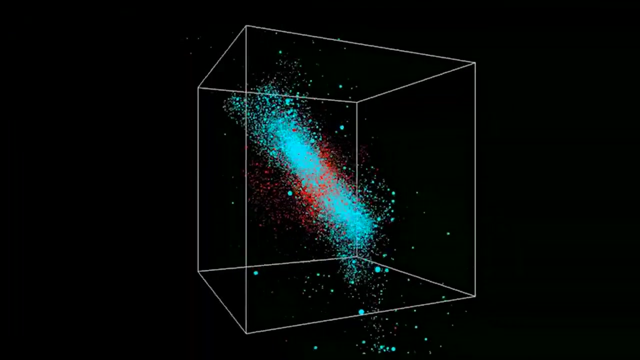 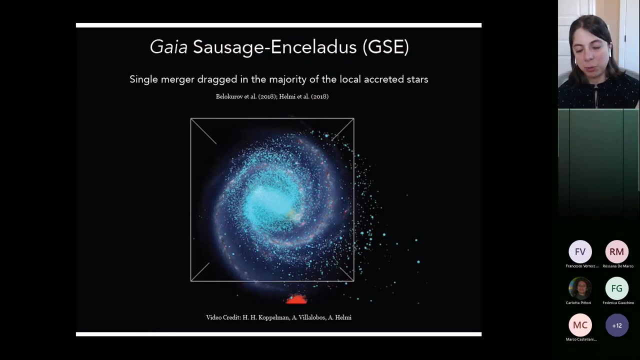 velocity direction, Next slide. So this was going to be a movie I'm showing, sort of proposing how that GSE merger would have taken place. So the, so we'll just skip that for now. But the identification of GSE which was made in some of the first papers, that 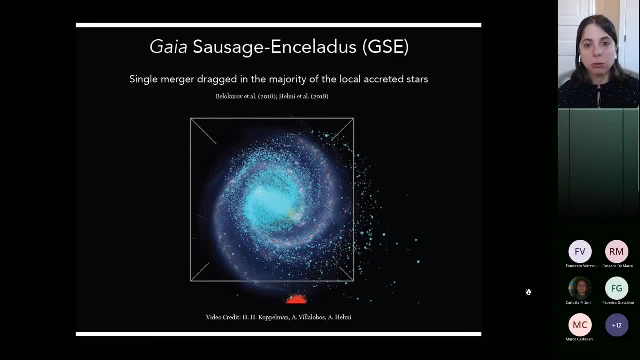 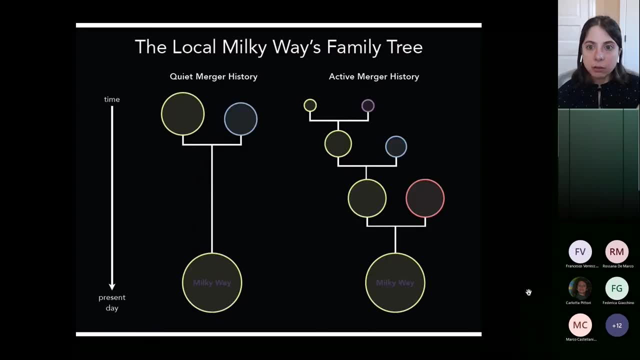 came out of from Gaia, Data Release 2 by Belokurov and then also by Helmy et al. Next slide Was a really important step in understanding the local Milky Ways family tree because it immediately ended up pinning down what is likely to be the last major merger that built up our galaxy. Next, 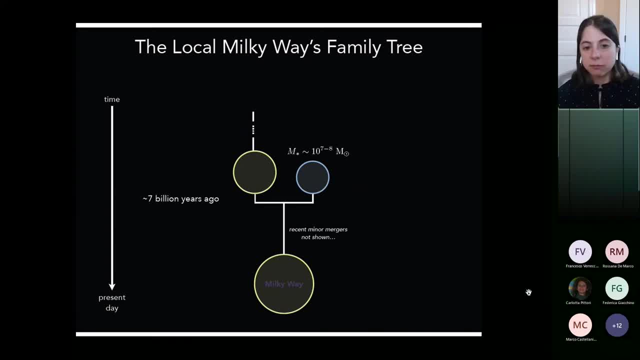 slide. So we've gone from like really not knowing what happened in this evolution to all of a sudden having pinned things down to a period roughly seven. That's definitely a tilde. It can range from like eight to ten Billion years ago, where a fairly massive system, this GSE galaxy, collided with our own and then 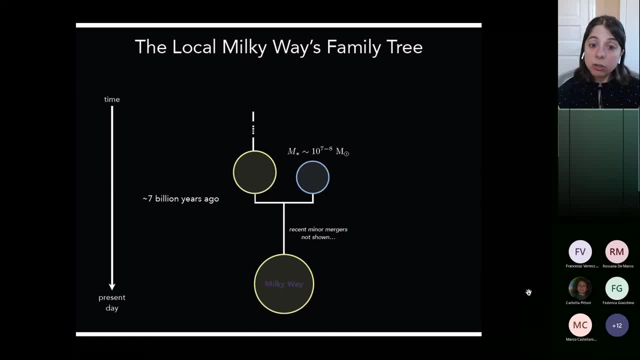 got completely disrupted. So it turns out that, you know, eight to ten billion years- giga years is- is roughly. it's not enough time for all of this material to have fully equilibrated by today, but it's also long enough that the material would be fully phase mixed and that we only really 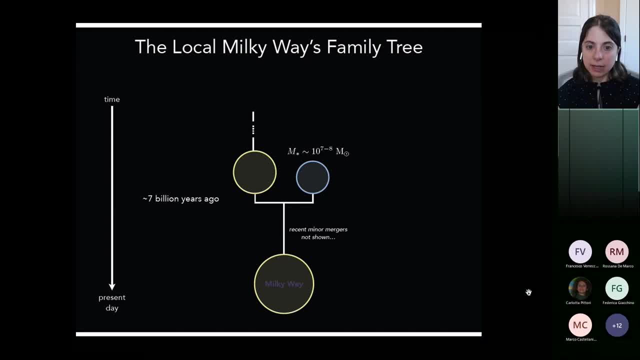 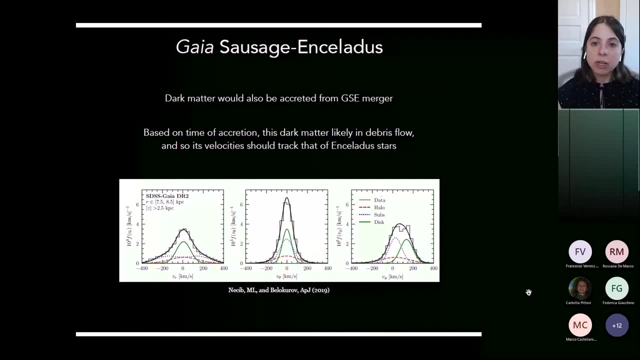 see it in its velocity properties Next slide. So the nice part of that is for this GSE merger, then we believe that it probably came from one of you know. when we look at in simulations that sort of corresponding mergers, this is precisely the class where the stellar tracers 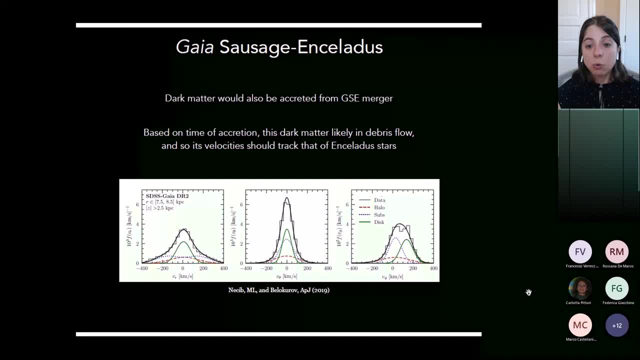 follow the dark matter distribution pretty closely So we can go in and do careful measurements of velocity distributions. Billion years ago we saw that the dark matter distribution was very, very important for the stars that came from GSE And and then infer from that that the GSE probably 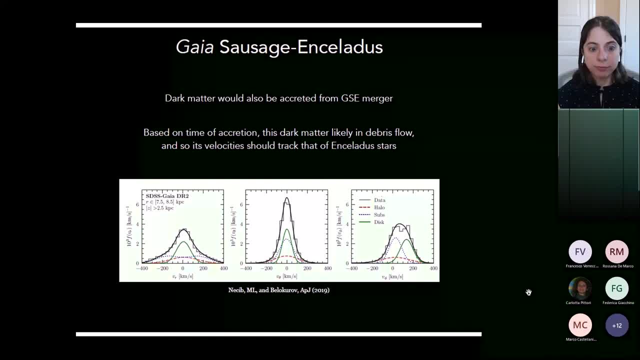 dumped a bunch of dark matter that followed that same velocity with the same set of velocities, And so these are just images of plots in radial phi and theta. velocities and spherical galactosectric coordinates of the the Enceladus stars are shown and dotted blue. 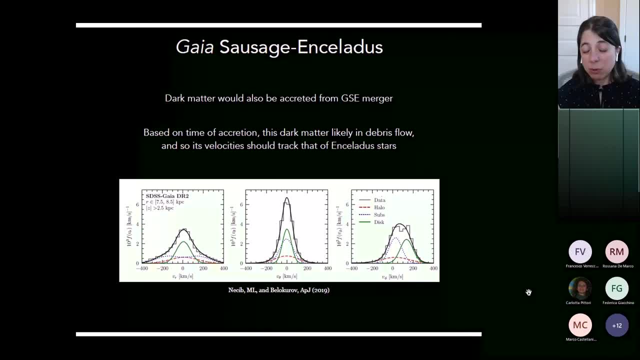 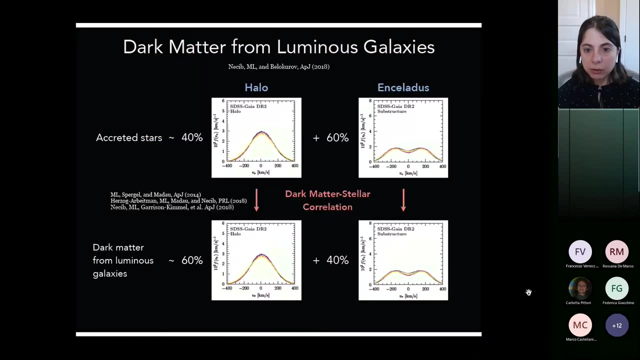 And so we believe, based off of what we've been learning from simulation, that the the dark matter from this Gaia sausage and the lattice would probably be following a similar kind of velocity pattern Next slide. So we can then go through an exercise of starting to actually build up a model. 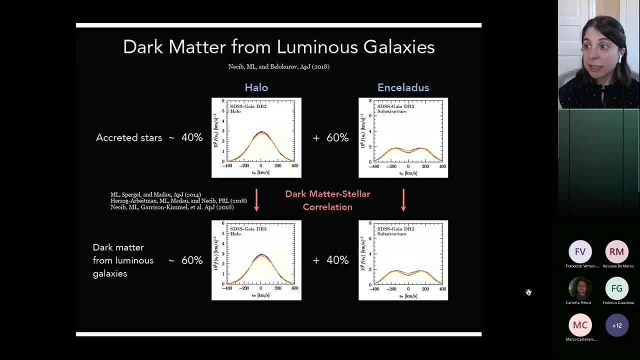 for the dark matter near the sun that would have come from luminous galaxies. This is actually a a pretty complicated extrapolation procedure to get these fractions correctly, So I'm happy to answer any questions about it afterwards. I'll just sort of summarize the results. 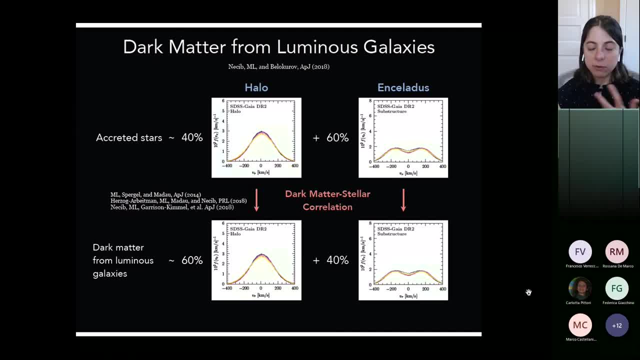 From the data, from the Gaia data, we can look at sort of the fraction of these GSE stars near the solar position. So there's about 60% there in GSE and about 40% that are coming from these old, really old mergers, And then, based off of that, we can extrapolate to the dark matter. 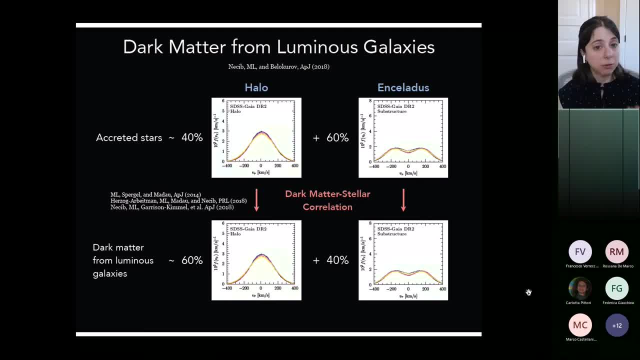 that about 60% of the local dark matter would be coming from the really old mergers and about 40% from GSE. So this is already telling us something about how to then build up and understand how that dark matter velocity distribution should be looking like near the sun. Next slide: 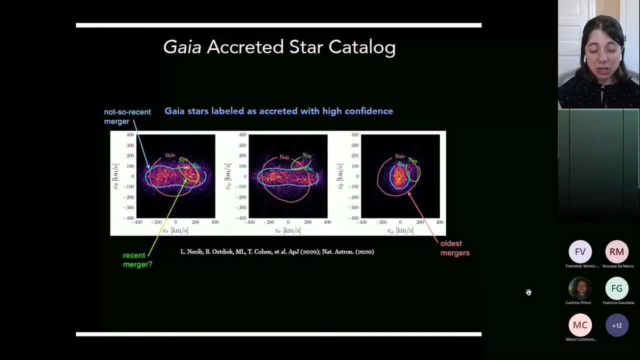 So there's one other piece here that I just wanted to talk about before concluding. It's the blob that's in green. So this was something that hadn't been identified before, and so we saw it for the first time. looking at this, accreted stellar. 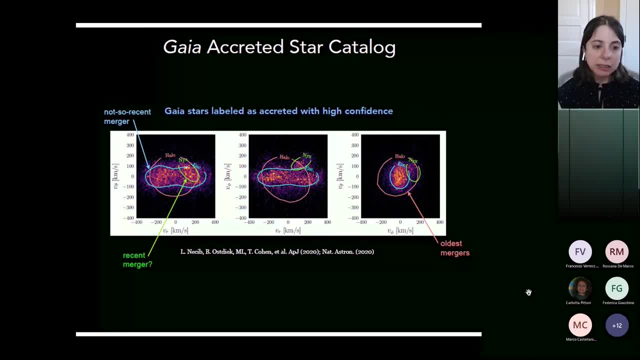 catalog. And it's curious because it has a very high radial velocity And it's also pro-grade, so it's more than just a very high radial velocity And it's also pro-grade. so it's more than just a very high radial velocity And it's also pro-grade, so it's more than just. 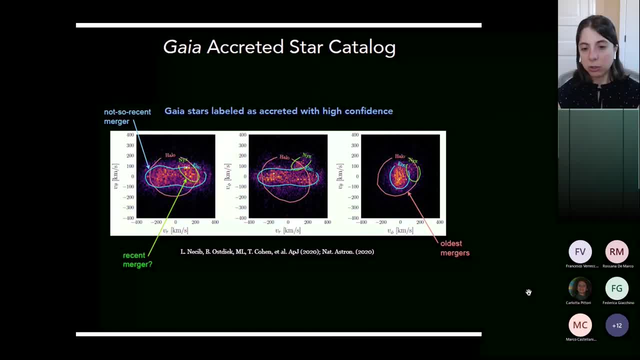 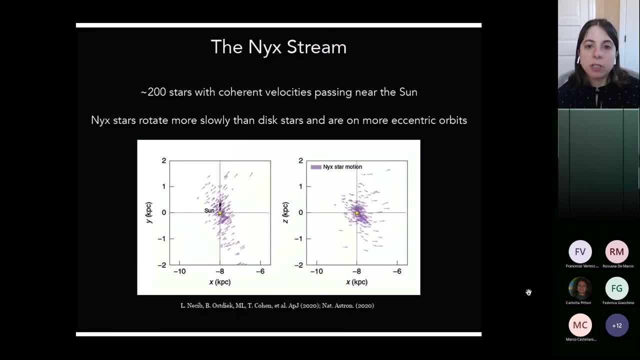 moving, essentially moving with the disk, but a little bit slower than the circular velocity of the disk Next slide. So we refer to this clump of stars as the Nix stream. There's a lot of them that are in this. It's about 200 stars And they have very coherent velocities, which you can see. 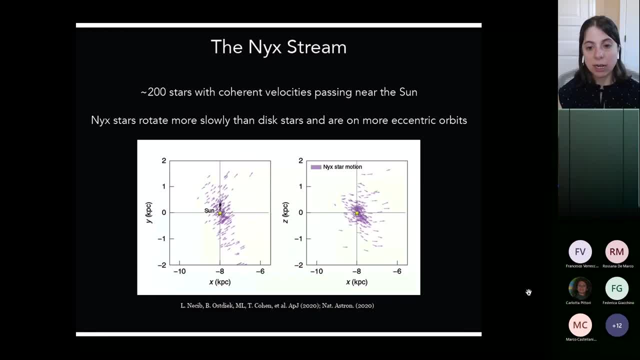 in this image here. So these are just the locations of the stars in x, y and z. The sun is indicated by the yellow star in the middle And the sun is indicated by the yellow star in the middle And and the arrows show the velocity for each of these stars And you can even just see by eye. 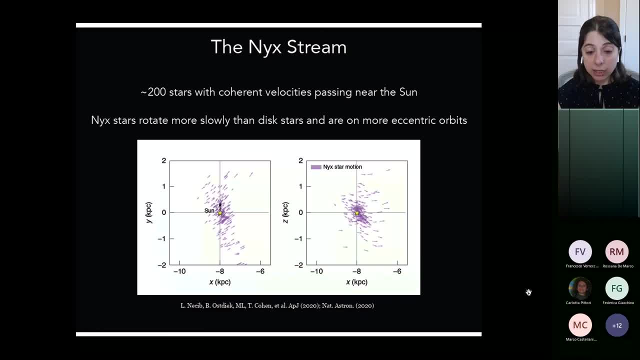 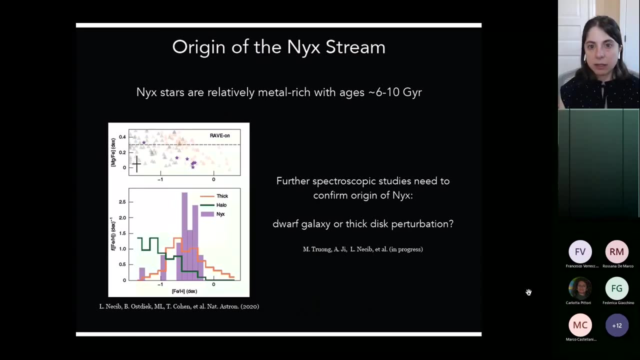 that it's very coherent. Their orbits are very eccentric And, like I said earlier, they rotate a little bit more slowly than actual disk stars Next slide. So there's an open question now on what the origin of that Nix stream is, And it's very complicated trying to figure this out because 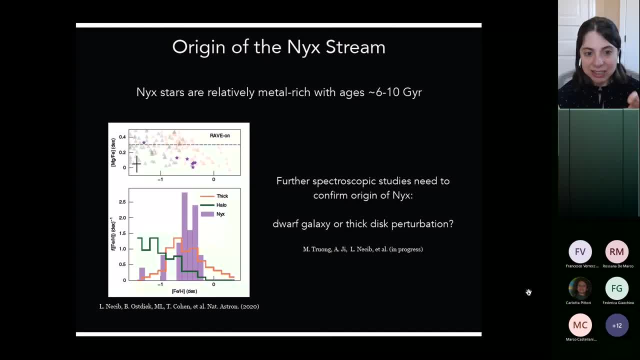 Nix is essentially embedded within the disk And essentially the big question is: is it actually a stream that came from a dwarf galaxy Or is it some kind of perturbation to the stellar disk in the Milky Way? And the one way to sort of be able to distinguish these two cases is by 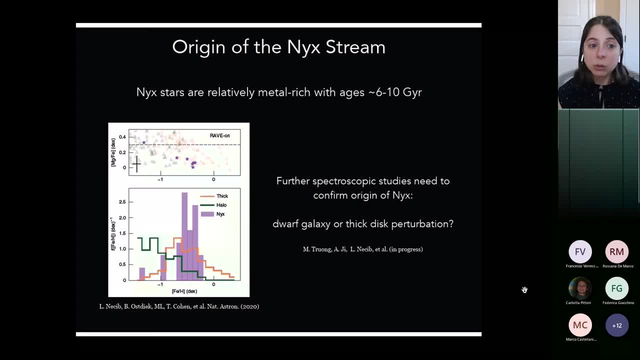 looking at the spectroscopy of stars that would belong to Nix, So looking at their chemical compositions, And when we first wrote this paper there weren't that many of them. So we're going to look at the spectroscopy of the stars that would belong to Nix And when we first wrote this paper. 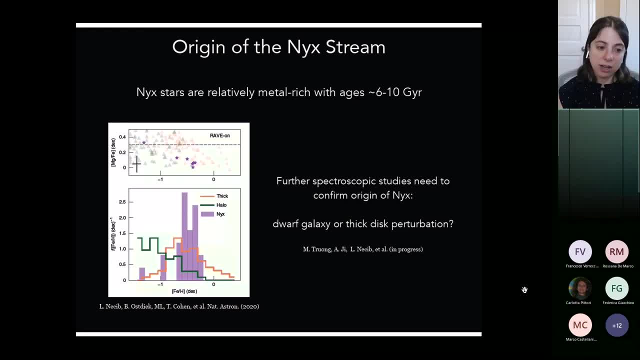 there weren't that many stars in the Nix subset for which we had a large amount of spectroscopy for, So that made it hard to distinguish. That is rapidly changing, which is great, because I think this is going to be sort of the key in understanding the origin of this Nix stream. I've highlighted 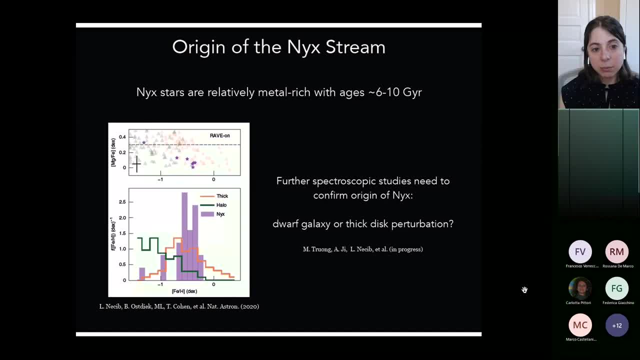 here some work that's ongoing by Alex Gee and Lina Nassib. They did some dedicated observations of Nix stars with the Magellan telescope that will hopefully be coming out this year. It was unfortunately delayed because of the pandemic, Next slide And actually just earlier this week. 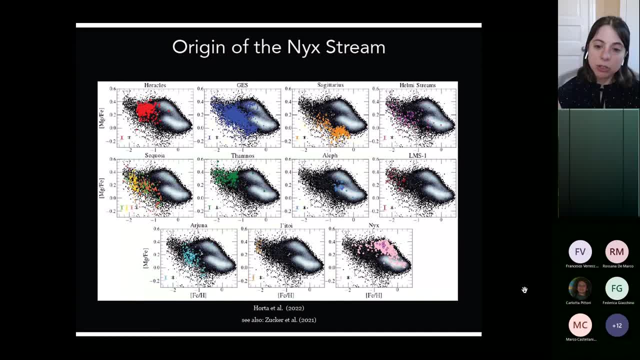 there was a study that came out from the Apogee survey looking at the chemical compositions of a variety of different substructures in the Milky Way, And Nix was one of these. So they're the bottom most bright panel shown in pink. So this is showing the metallicity distribution of 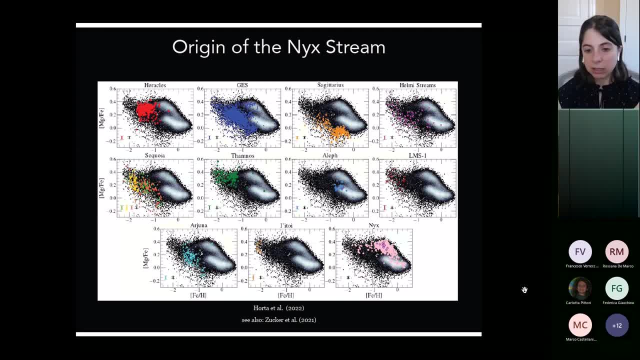 the Nix stars. So iron over hydrogen is on the x-axis, and on the y-axis is magnesium over iron. And just to kind of give you a sense, the background, which is in gray and black, is an expectation of where the in situ disk stars should be. And so, from this sort of initial, 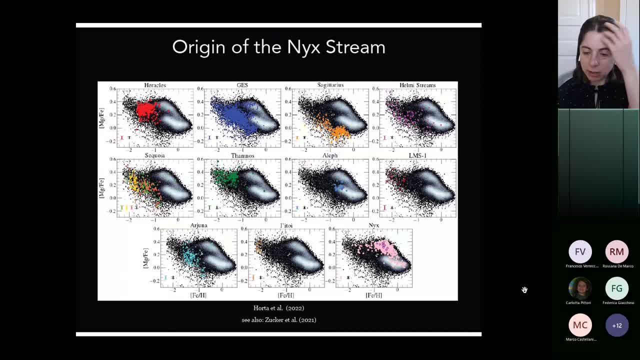 work. it does seem like Nix might be coming from the high alpha stellar disk, But it hasn't been, So this is a very significant tail that goes down to low metallicities And painting a picture that makes these results consistent with the unusual kinematics of Nix, I think still. 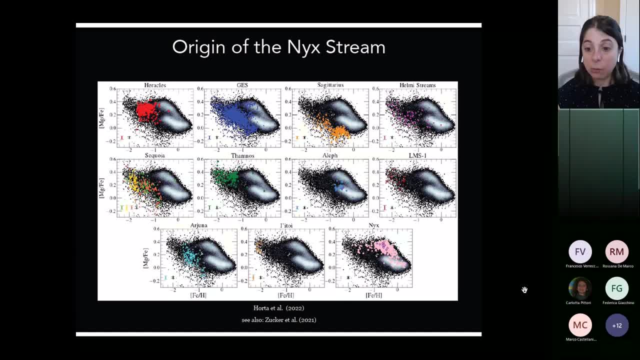 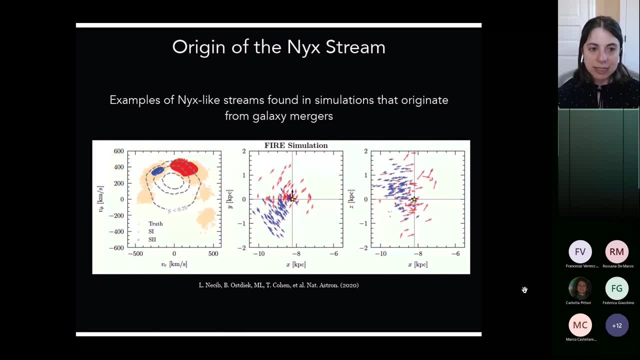 requires some more work to understand more fully. Next slide, And since I'm running out of time, I won't go through this in detail, But just to say that we've looked in simulations to see if we could find structures that are similar to Nix. And we do see them there, And they come from dwarf galaxies. 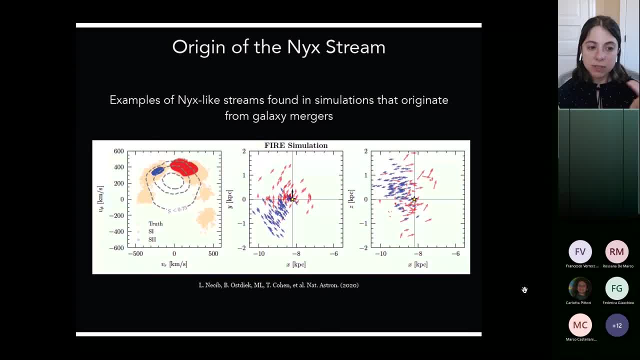 And so one of the things that we're working on now is sort of digging into these simulations and really kind of understanding exactly if it is coming from a dwarf galaxy, what would that kind of structure look like? Is it consistent with what we're seeing in the data? Can those dwarf 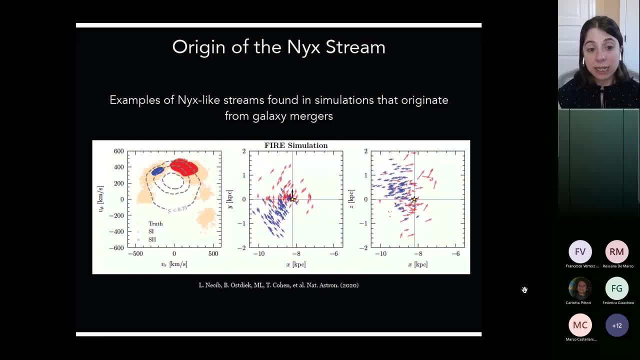 galaxies be creating a perturbation in the thick disk And maybe that's what we're seeing in Nix. So this is just meant to just highlight the fact that there's sort of a big open question, I think, on what's going on here And with further spectroscopy studies and also looking more. 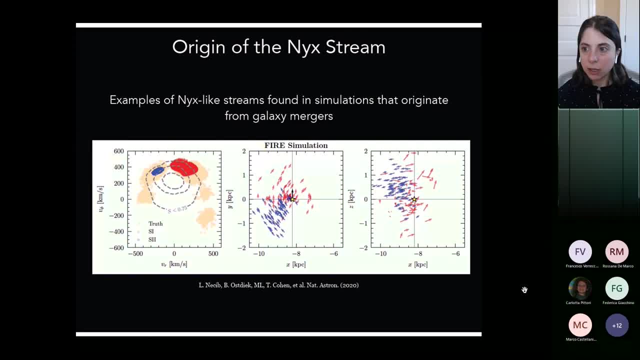 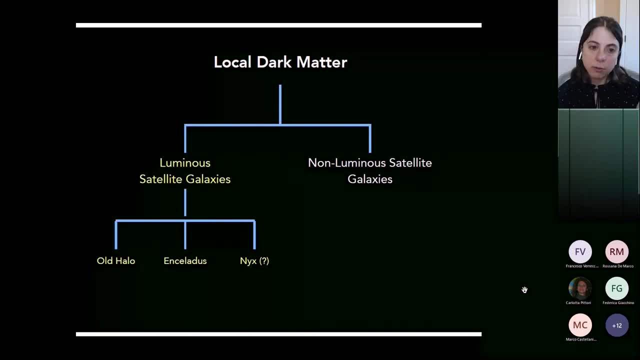 into the simulation. we'll hopefully be able to clarify this better moving forward Next slide. So this is just meant to kind of summarize where we're at now in understanding the contributions of local dark matter coming from luminous satellite galaxies, From the Gaia data. we 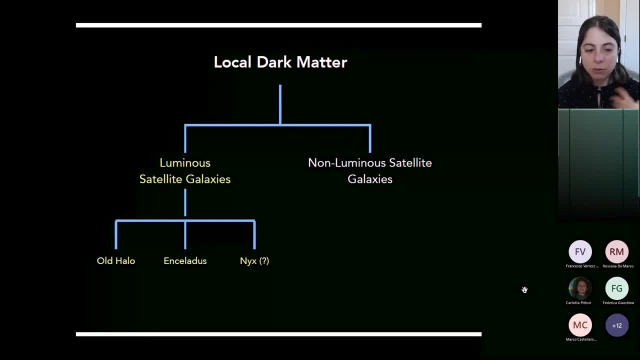 do see that there is a component of the dark matter in the Sun that would have come from very old mergers, So galaxies that would have come into the Milky Way before Redshift 3.. There is a significant amount of the dark matter near the Sun that is coming from this GSE merger, So this 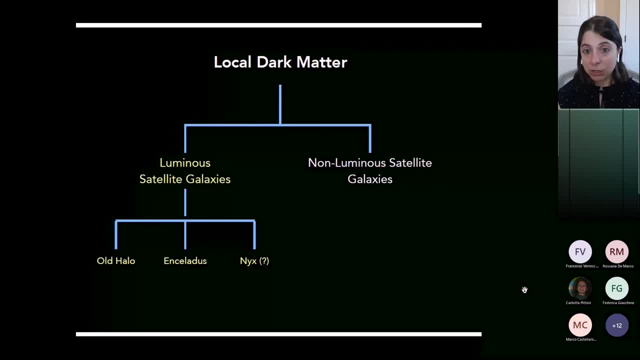 the last major. it's referred to often as probably being the last major merger for the Milky Way And possibly Nix. if Nix is coming from a dwarf galaxy- Nix is not coming from a dwarf galaxy- then it wouldn't be contributing, So that's still a big 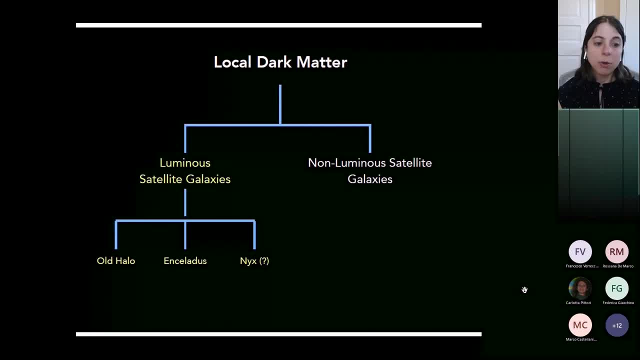 question mark that we need to sort out. But already understanding this old Halo plus GSE piece is a big step forward. If it was only the old Halo piece, then the Maxwell-Boltzmann distribution is a good model, But now that we know that GSE is contributing dark matter near the Sun, 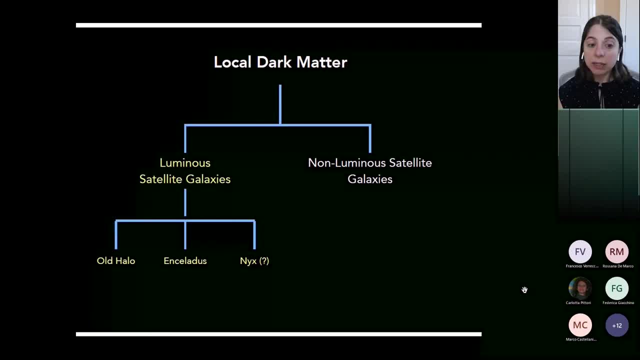 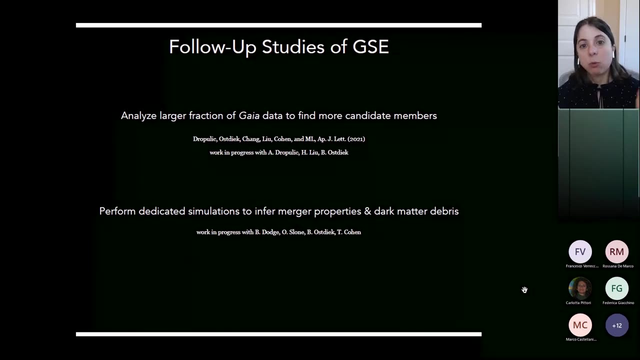 we know that that Maxwell-Boltzmann model is not fully correct and that there's additional contributions, at the very least the contribution coming from the GSE Next slide. So I had a few slides here just talking about work in progress, Since I'm already running late. 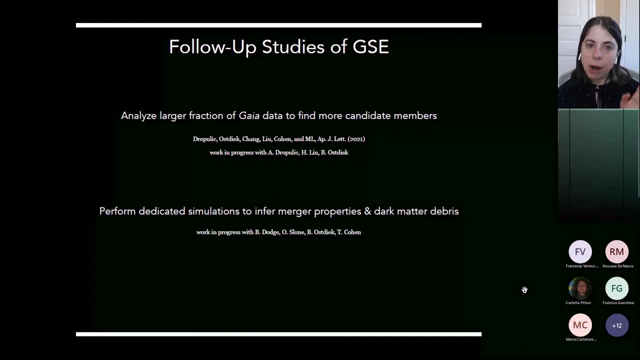 since we started with some delay because of the technical difficulties, I'll probably just stop here, But just let me just share a few words on kind of where we're taking this, Because we've learned now that there is a significant amount of dark matter near the Sun. there is a significant 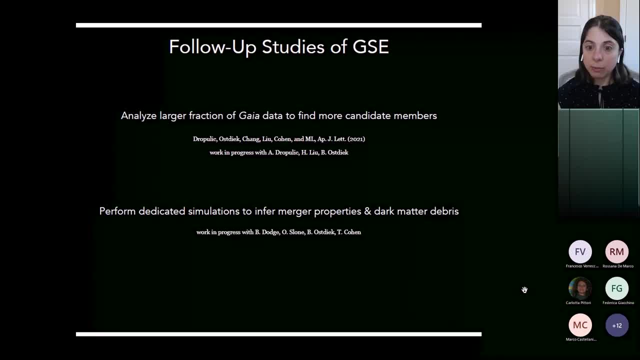 contribution coming from this GSE merger to the local dark matter. We definitely want to understand the properties of that much better and try to even improve the modeling of the velocities of the dark matter that would be expected to come from the GSE merger. So there's a few avenues in. my research group that are trying to answer this question. One avenue is trying to figure out whether or not we can analyze a larger fraction of the Gaia data to find more candidate GSE stars. The goal of that would be to essentially remove statistical uncertainty and build a better model. 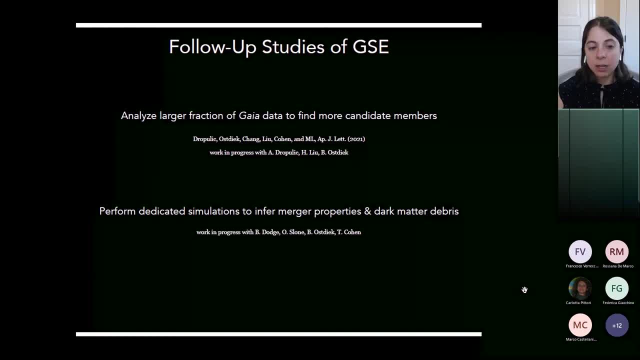 of the velocity distribution of the local GSE stars. And then the second piece is actually running dedicated simulations of GSE type mergers to really identify the properties of the GSE galaxy, so its original mass, its original in-fall time, its orbital properties. 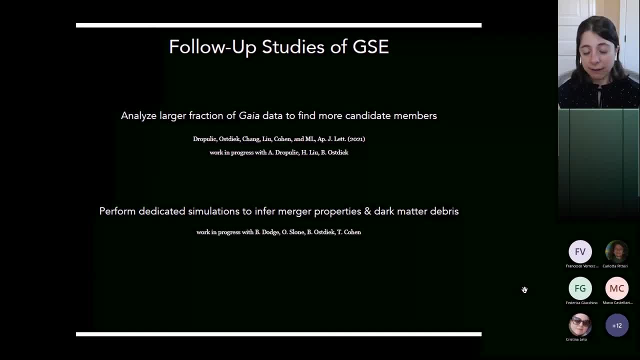 That's really key. key if we want to make sure that we definitely understand the dark matter that would have come from the GSE and the properties of that dark matter today. And getting these simulations right is really tricky because the GSE merger is quite significant. It was a major merger of the Milky 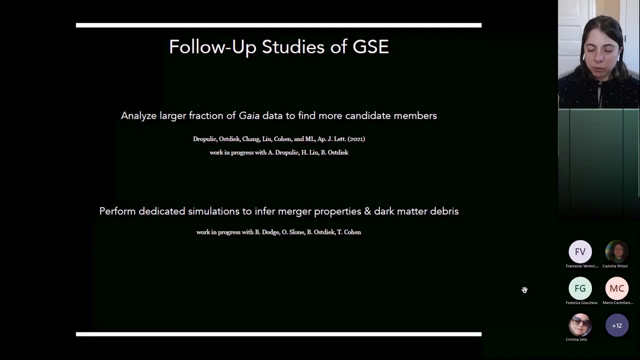 Way. So as it was falling in, it was perturbing the Milky Way stellar disk, It was causing it to tilt and precess, And all of that behavior needs to be properly accounted for if we want to make sure that our predictions for the dark matter debris from GSE- are spot on. So we also have some. 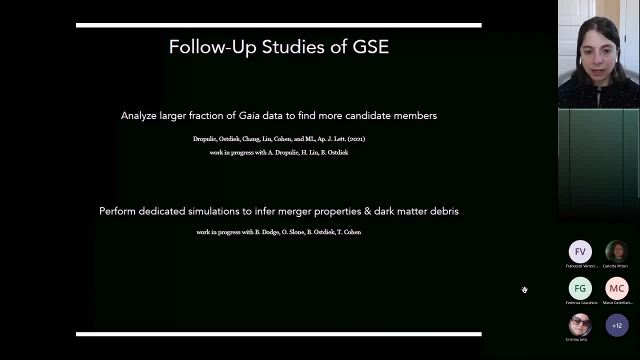 ongoing work that's trying to get that in place. So I'll skip the next few slides, which is just sort of going into more detail on this, And then I'll conclude. I think it's like three slides that I'll skip here.